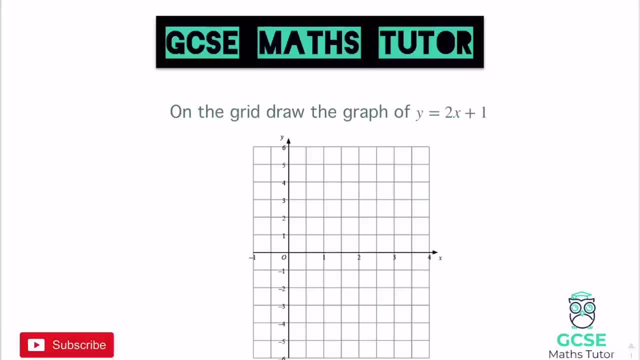 make some notes and we're going to get started on this one. So this first one says on the grid: draw the graph of y equals 2x plus 1.. Now there's lots of ways of doing this, but essentially it's. 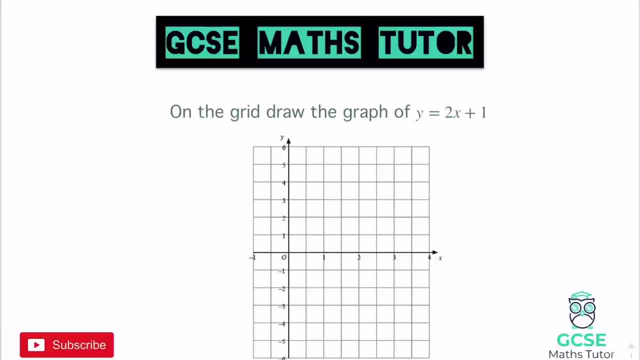 just about understanding what this actual line equation means here. So we know, hopefully, that all line equations need to be in this form: y equals mx plus c. Okay, so y equals mx plus c. Again, in this line equation, m represents the gradient, which in our line equation here is the: 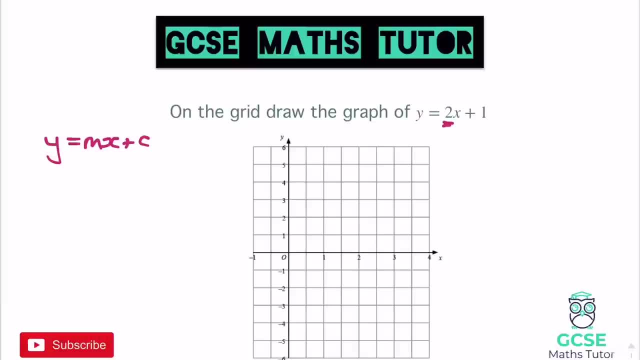 number 2, so we have a gradient of 2, and c at the end there represents the y-intercept, which for us here is positive 1, so we've got a y-intercept of positive 1.. Now, in terms of what that means, 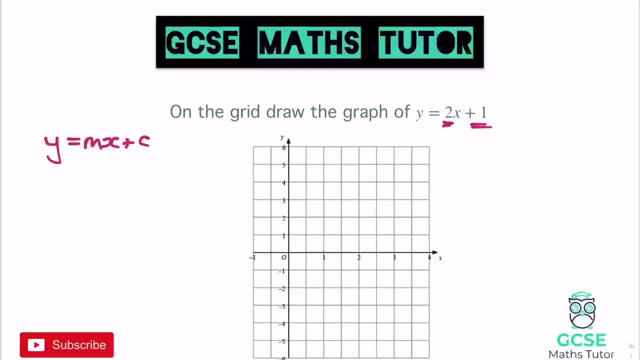 the graph's going to look like. we know it's going to cross through positive 1 on the y-intercept, which is right here. Okay, I'll try and mark that on. There we go. So we know the line's going to go. 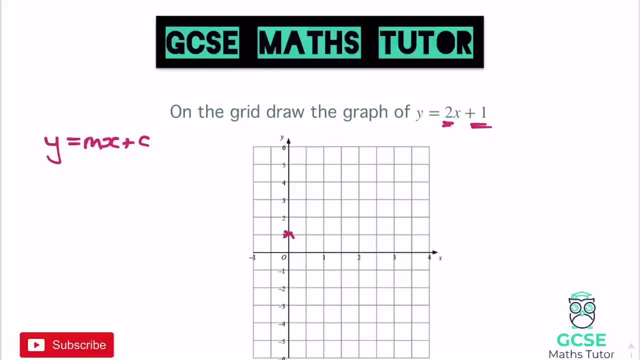 through this point and all we have to do is figure out where all the rest of the coordinates are. Now, in terms of y equals 2x plus 1, remember, x and y relate to the x and y coordinate. so all that we need to do is actually pick some x coordinates. Now, if you have a look on the graph, you can see. 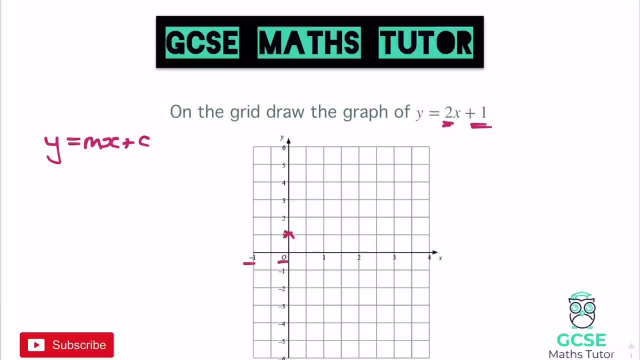 there's lots of x coordinates here. We've got minus 1,, 0,, 1,, 2,, 3, and 4 at the end there. Okay, so all we have to actually do is pick them, double them and add 1, and that'll tell us where. 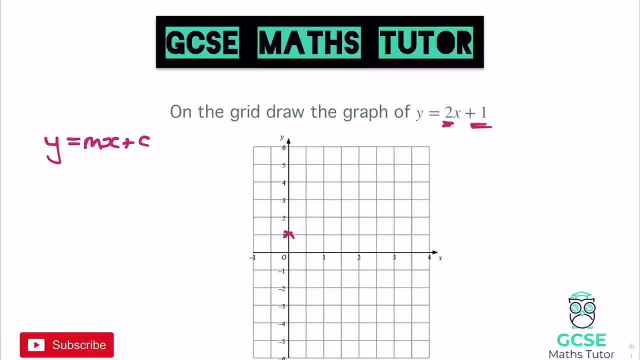 the corresponding y coordinate is, And we can do that using a little table, and you don't have to use a table, but just tidy it up a little bit. if we just make a little table here, Sometimes you'll need a table, but it's quite unlikely that you'll be given it. So we've got some x coordinates. 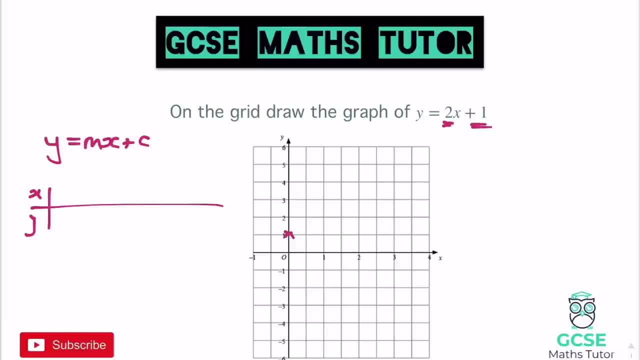 and we've got some y coordinates we need to find. Now for x. we've got starting at minus 1, and then it goes 0, and then we've got up to 4, so 1,, 2,, 3,, 4.. So if we start with negative 1,, 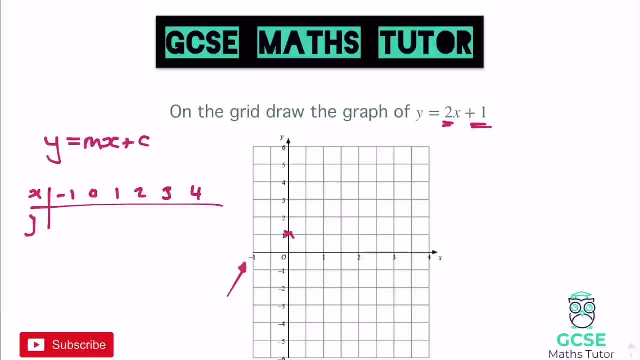 this one. here we need to double that and add 1.. Now I'm going to just sub that into my little equation up there. so y equals 2x plus 1, so it's 2 lots of minus 1,, 2 times minus 1, and then add 1.. 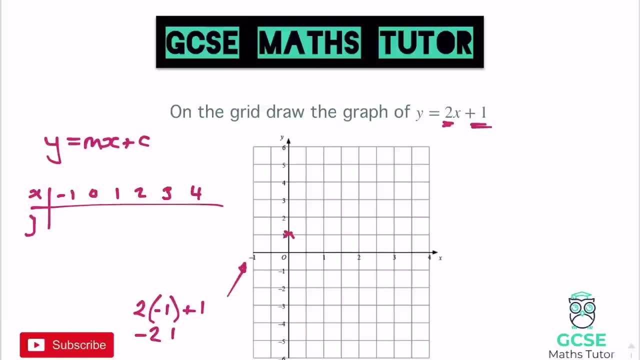 And if we double negative 1, we get negative 2, add 1 to that gives us negative 1.. So our first y coordinate there is negative 1 as well. so minus 1,, minus 1.. And we can plot that if we want straight. 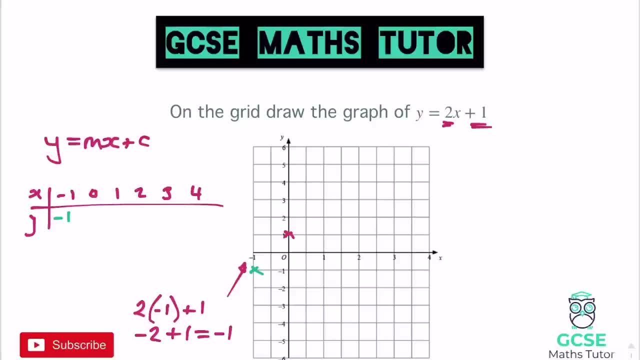 away There. it is minus 1, minus 1.. Moving on to the next one, what do we have for this next one? We have the x coordinate of 0. So if we just, without doing all the working out for all of 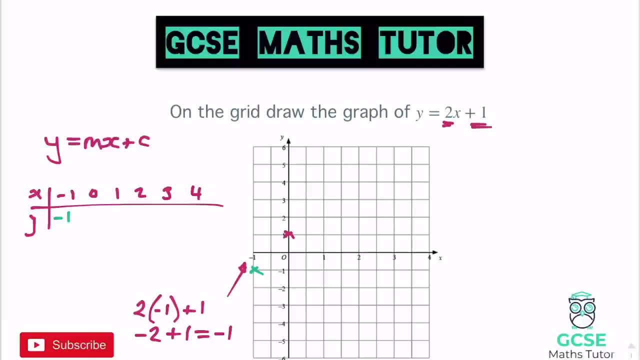 these. let's double 0, it's 0, and add 1.. So 2 times 0 is 0,, add 1 is 1.. And if we carry on doing this for the next one, so when x is 1,. 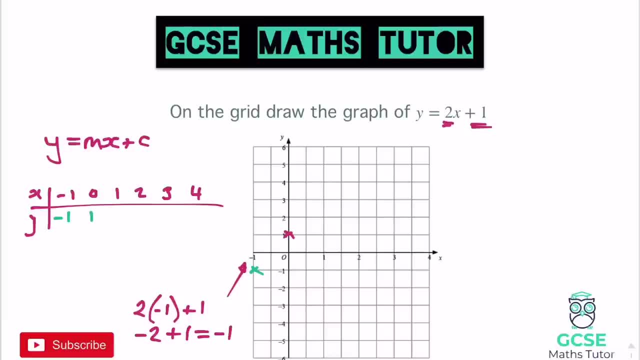 double 1 is 2, and then add 1 is 3.. So double 1 is 2,, add 1 is 3. And you can start to see there's a little bit of a pattern emerging. Okay, between all of these points, if you have a look from minus. 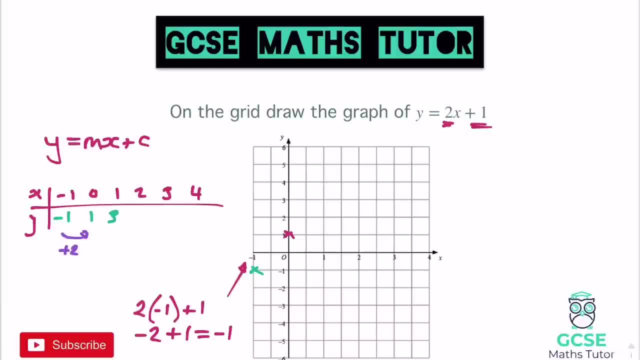 1 to 1,, that is adding 2.. From 1 to 3,, that's also adding 2.. So actually all we need to actually do is keep adding 2.. So add 2 to 3 is 5,, add 2 again is 7, and add 2 again is. 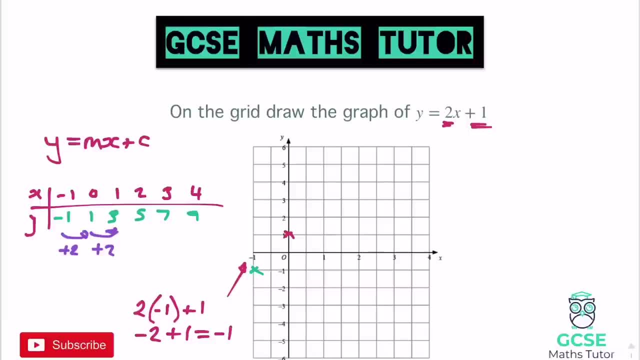 9. And then we can go ahead and plot as many of these as we can. Obviously, we can't do them all here because the graph is not big enough, But for the next one let's have a look. 1 to 3 is there, and 2 and 5 is there. Okay, so there are the points we can plot. We could actually plot it up to this point here. I don't have the ஆ 17.. But once we've done that, we need to do the next calling and we're going to have a solving just to add 2 to 3.. Let's come back again: 20 to three, We add 1 to 3 is 5,, 7 and add 2 again is 9.. Add 2 again is 9, and add 2 again is 9.. And then we can go ahead and plot as many of these as we can. 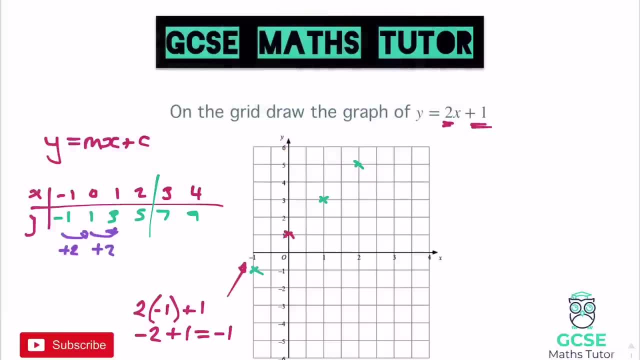 But once we've done that, all you need to do is grab a pencil, grab a ruler and join it up nice and straight, all the way through the graph, unless it states otherwise. So, with your ruler, nice, straight line, going all the way through and extending it up to the edge of the graph there. 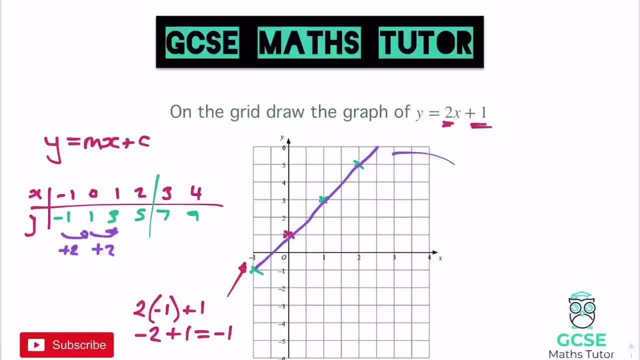 There you go and that is your line, And it's always good practice just to label it. You don't have to, but you can just label that as the line y equals 2x plus 1.. It just helps if there are multiple graphs or multiple lines on the graph, but you don't have to label it unless you're asked to. 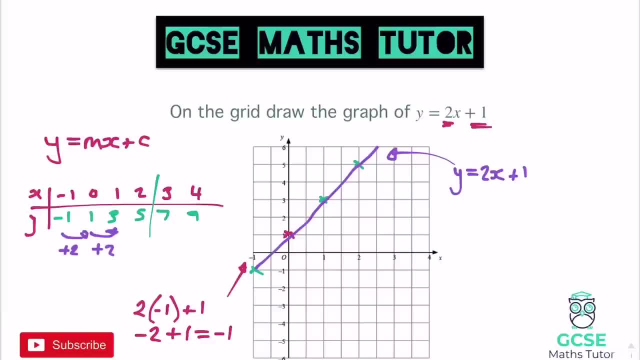 Okay, but there you go. y equals 2x plus 1.. And there are other ways of drawing this and it just comes to having an understanding of the equation there. So we already talked about one of them. the fact that it starts on the y intercepts up plus 1.. 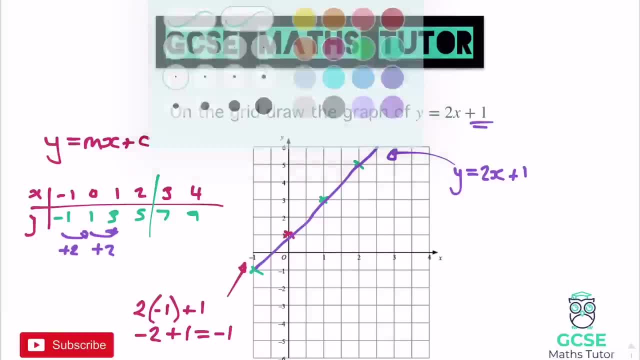 And then the fact that it has a gradient of 2 just means that for every step across from a point on the line. so if we look at this as I know, it's two squares there. you've got to be careful of the scale. 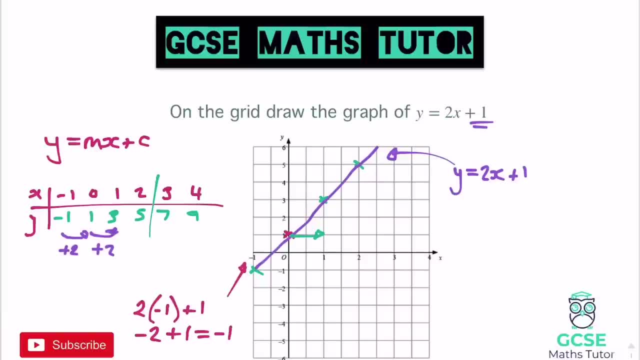 but that's 1 across, going from 0 to 1. And if you have a look, it goes up from 1 to 3.. There you go, So it has a rise there of going up 2 for every 1.. 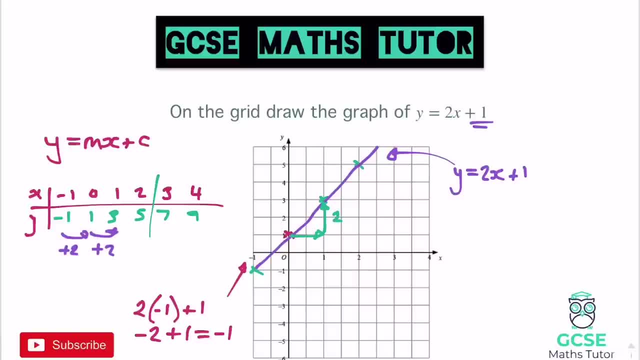 And you can always draw this in. It's a way of understanding it as well. So it's 2 there and 1 here. Every 1 across it goes up 2.. And that's what a gradient of 2 actually means. 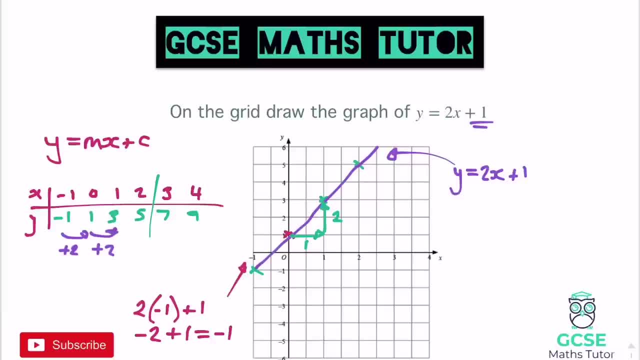 It means for every 1 step across, it goes up 2 steps, Even though the scale is slightly different here. it's 1 in terms of the numbers across and 2 in terms of the numbers going up, And that is what a gradient of 2 actually represents. 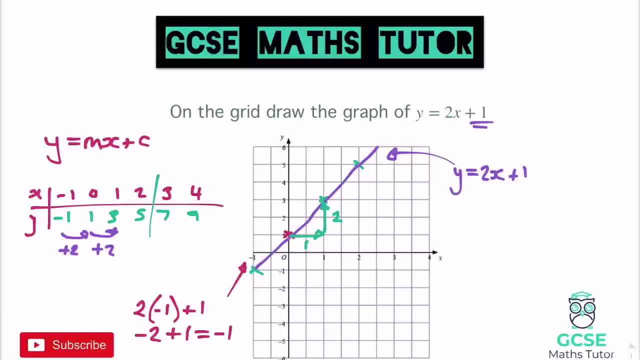 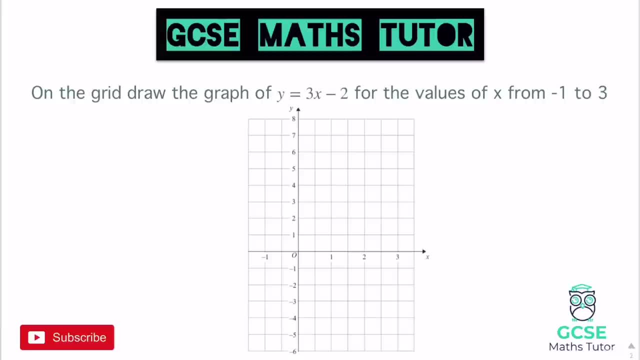 But it's best bet is just to draw the little table out and then get all your numbers nice and neatly drawn in. Okay, let's have a look at one more. Okay, so on the grid, draw the graph of y equals 3x minus 2.. 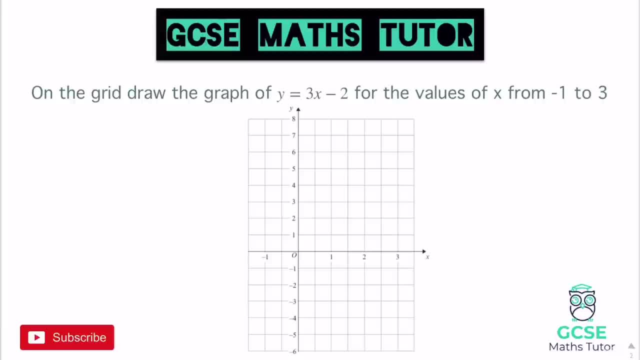 Okay, this time it says for the values of x, from negative 1 to 3.. And again that's what we actually have on the graph. there We have from negative 1 over here, going across from 0,, 1,, 2, and finishing at 3.. 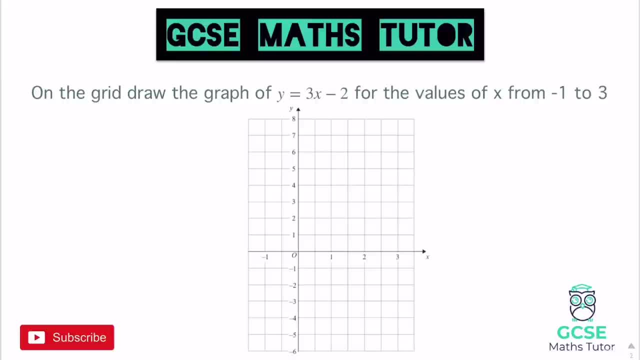 So we can use all these x values to draw our little graph. And again, I'm just going to draw a little table for this. But again, thinking about this equation and what it actually means, it has a y-intercept there at the end of negative 2.. 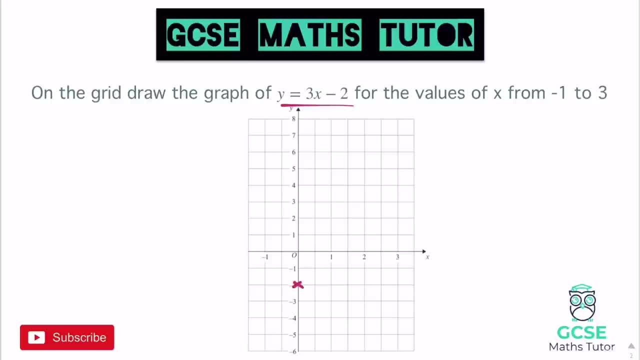 So we know it's going to cross through this coordinate here And it has a gradient of 3.. Which, in terms of just drawing a pattern, if I was to show you how I would actually draw this if we go across one square. so that's 1 there. 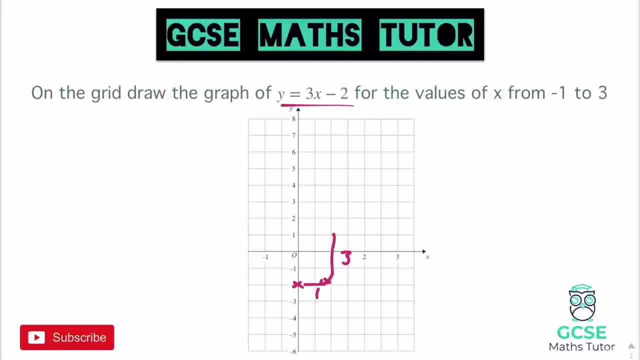 and then go up 3, again just being careful of the scale there. that's where our next coordinate is going to be, right there, Okay, but we'll see that when we actually draw the graph. But you can actually just do this following the pattern. 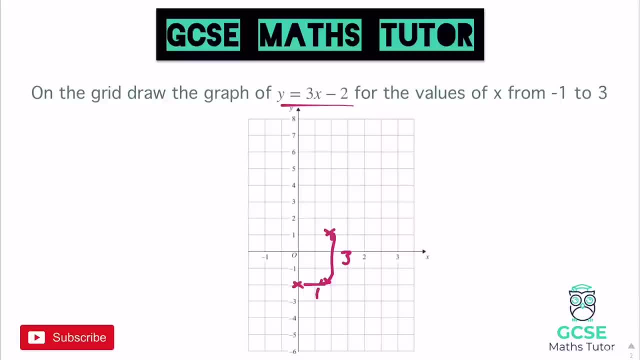 It's not going to help with the progression of this topic, but it does help make these ones nice and quick. You can just go across 1, up 3, cross 1, up 3. And you can just draw all these points in and join them. 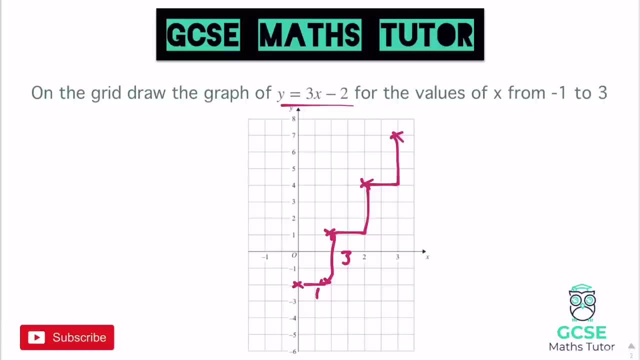 Okay, so this is what the graph is actually going to look like, And if we go across 1,, down 3,, there we are, there's our next one. So we could actually just draw this straight in, And it's a nice quick way of getting these drawn. 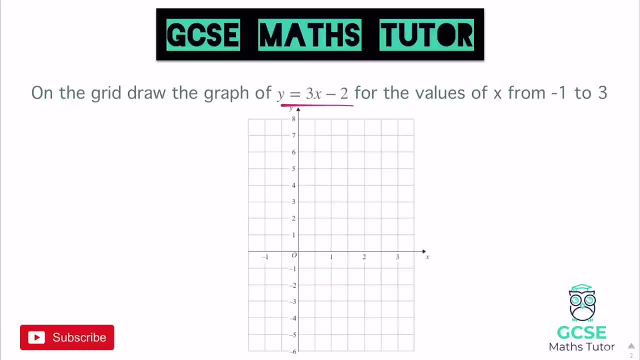 But I'm going to get rid of that because it's not going to help us really with understanding this at the moment. So if I draw my x and y coordinates, x and y and this one is 3x minus 2.. 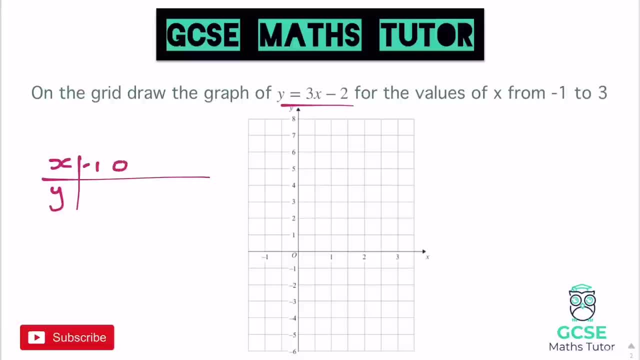 So it says from minus 1 to 3, so minus 1, 0, 1, 2, 3.. And again, just draw this, Just subbing the points into the equation. So if I start with negative 1 again, let's just do this one to start with. 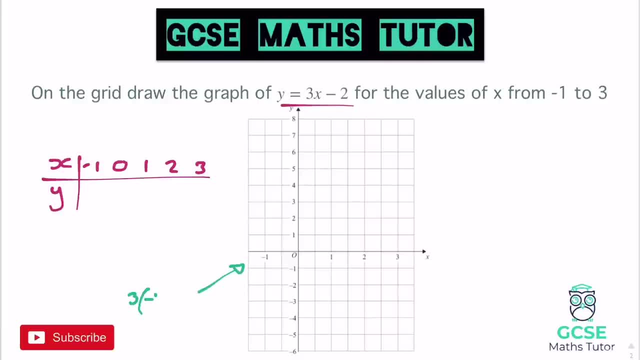 So for minus 1, we have 3, lots of minus 1.. And then take away 2.. 3 lots of minus 1 is minus 3.. Take away 2 is minus 5.. There we go. so minus 1 is all the way down here at minus 5.. 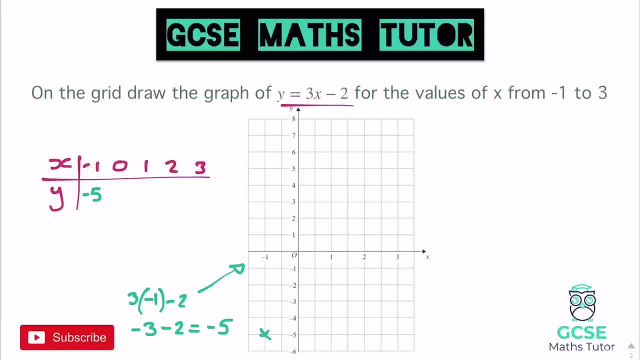 And we can put that into our little table. It's up to you if you want to draw the working out for all of them. I'm just going to follow this in my head now. So from 0,, let's triple, that is 0.. 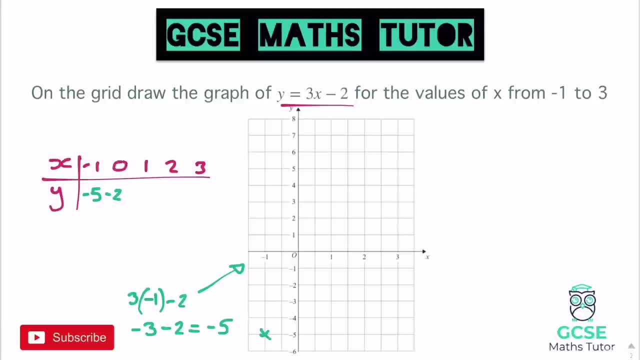 Take away, 2 is negative, 2.. There we go And again we can start to look at the pattern here And you'll notice it goes up by again this gradient, which is 3.. It's going up in 3s. 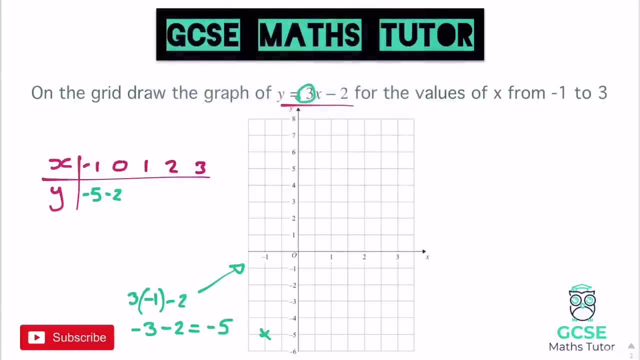 So if we just keep adding 3 each time, because it's just a bit of a sequence here, a bit of a pattern, Just plussing 3. And then again add 3 for the next one And just continue that little pattern, and that's fine, 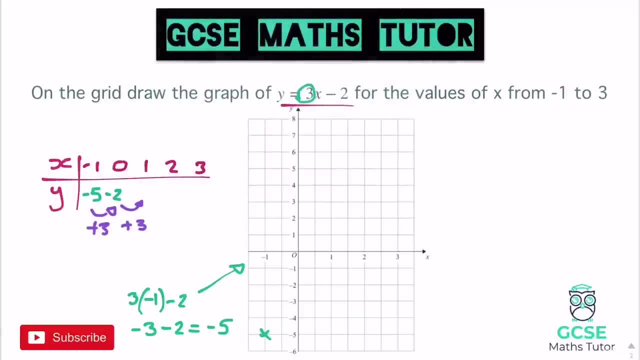 That's a nice quick way of getting these drawn. So add 3 to minus 2 is 1.. Add 3 again is 4.. And add 3 again is 7.. And then plotting all of these, So 0 minus 2, and there's that minus 2 that we knew we were going to get. 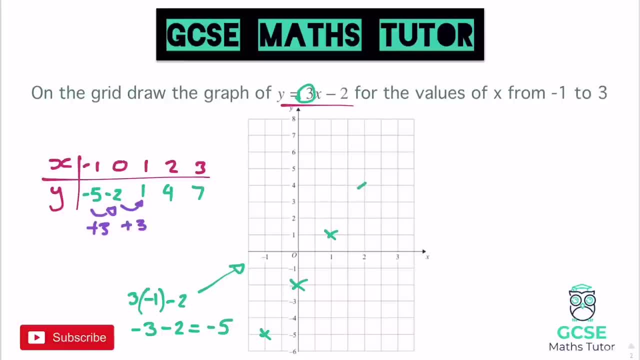 1 to 1.. 2 to 4. And 3 to 7.. There we go, Right. So this actually does say: draw it from the x values from minus 1 to 3.. So I am going to start from the 1 on minus 1.. 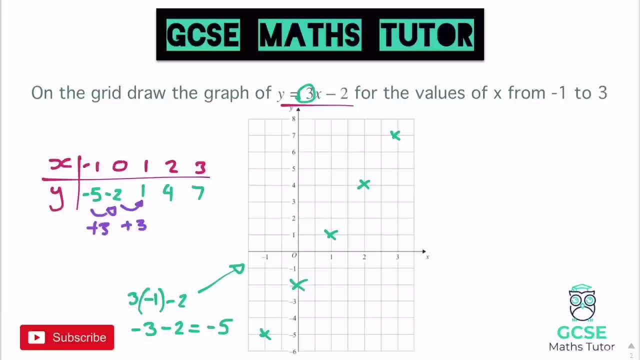 I'm going to connect it with a ruler and a pencil, if you're doing it on paper, up to the final point. But I'm not going to extend it this time because it just says to draw it between those two x values. 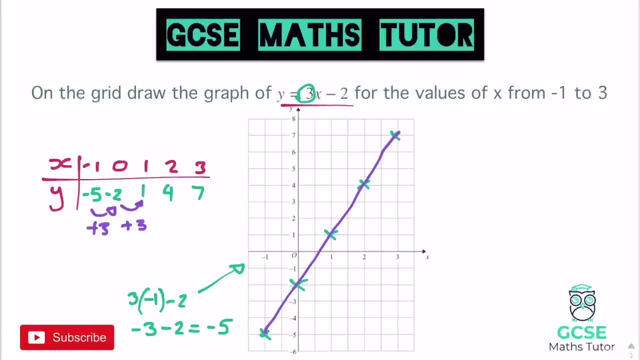 Okay, so I don't need to extend it beyond the points. You don't need to label it, but it's you know. if you want to label it, that's absolutely fine. You can just label it as: y equals 3x minus 2.. 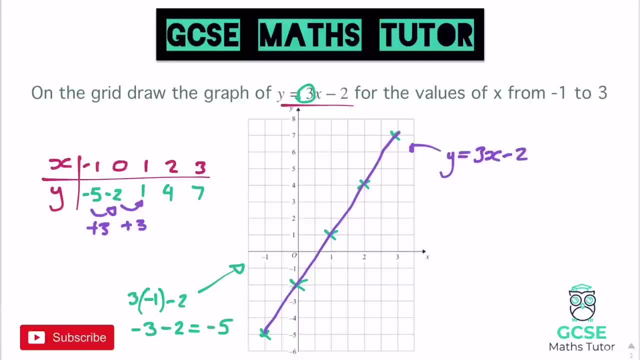 There you go, But don't feel that you have to do that. It's not, you know, unless you're explicitly asked to label it, you don't have to, Right? Okay, Here's something for you to have a go at. 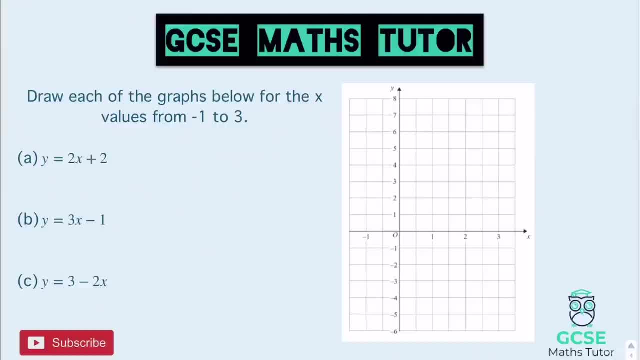 Okay. So obviously this does require you to actually draw some lines on a graph, So feel free to just pause the video and draw this graph out to the side. Okay, On the y-axis going from 8 down to negative 6.. 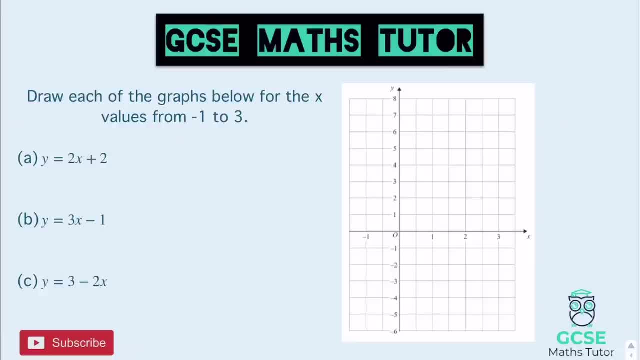 Okay, And on the x-axis, going from negative 1 to 3.. Okay, So we're going to be drawing these graphs in just a second, But there are three line equations there, So I would encourage you to draw a little table for each one. 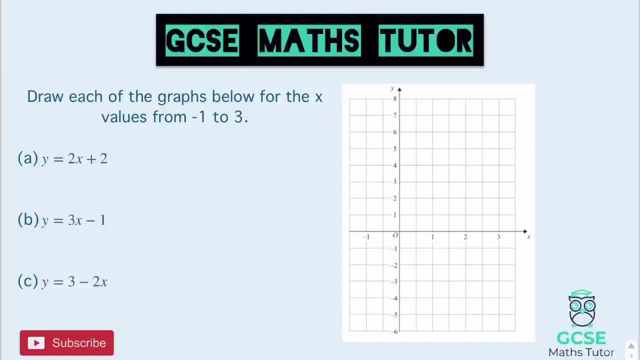 Have a go at drawing all three of them. Draw them on the same graph, Okay, And just label them up separately, And if you pause the video there, we're going to go over the answers in a sec, Okay, So the first one, part a. 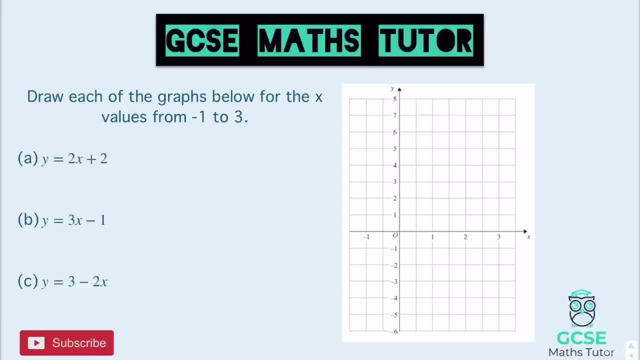 Right. So for all of these we're going from minus 1 to 3.. So if I draw myself a little table x and y From minus 1, 0,, 1,, 2,, 3.. So this one's double it and add 2.. 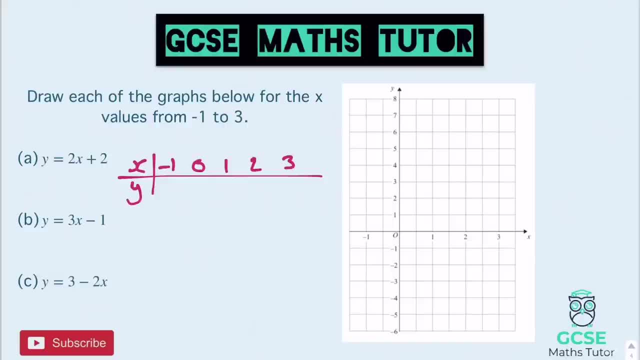 So negative 1 doubled is negative 2.. Add 2 is 0. And then it goes up into so 2,, 4,, 6,, 8.. And we can plot this on. So negative 1 to 0,, 0 to 2,, 1 to 4,, 2 to 6, and 3 to 8.. 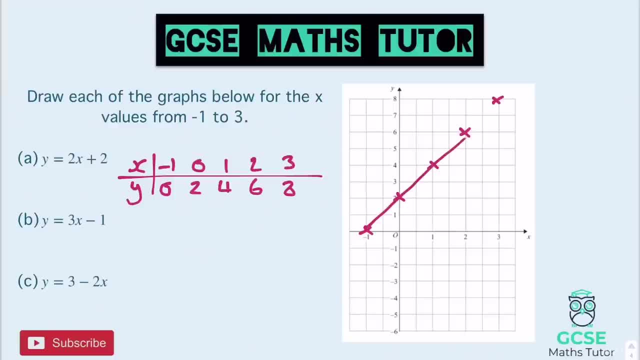 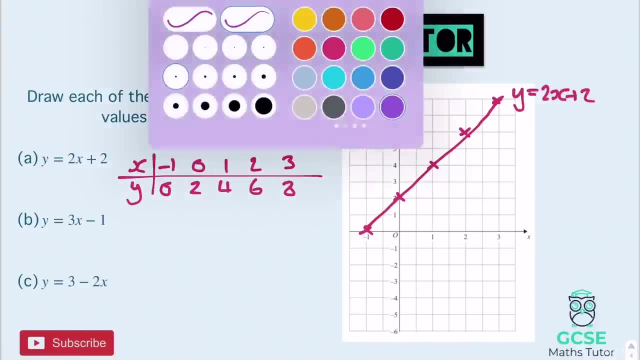 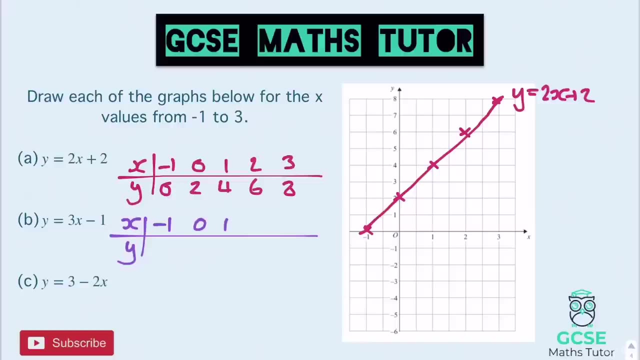 There we go, And that is our first one. Let's join that up. There we are, And that is our y equals 2x plus 2.. Onto the second one, Drawing another table, again X and y, And again minus 1, 0, 1, 2, 3.. 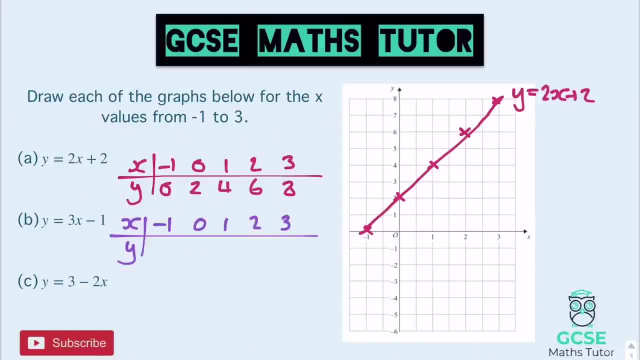 This time we're going to times it by 3 and take away 1.. So negative 1 times 3 is negative 3.. Take away 1 is negative 4.. And this one's going up in threes, So negative 1,, 2,, 5,, 8.. 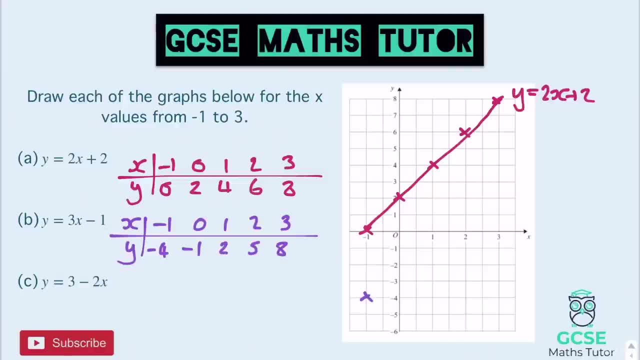 So negative 1 to negative 4 is here, 0, negative 1 is there, 1 to 2 is here, 2 to 5 is there And 3 to 8, again is finishing on that same final point as our last one. 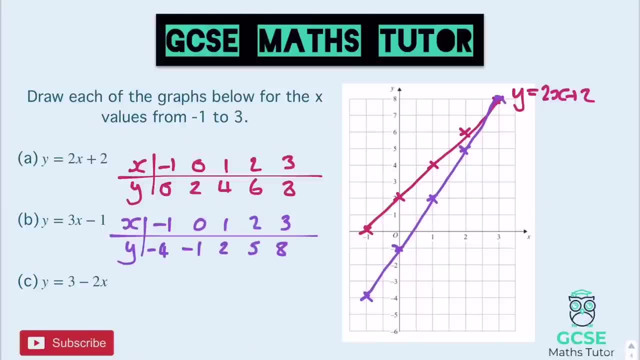 Nice and neat with the rule and the pencil joining that up, There we go. So that's our line. y equals 3x minus 1.. And then for the final one, here let's have a look. This one's a little bit trickier. 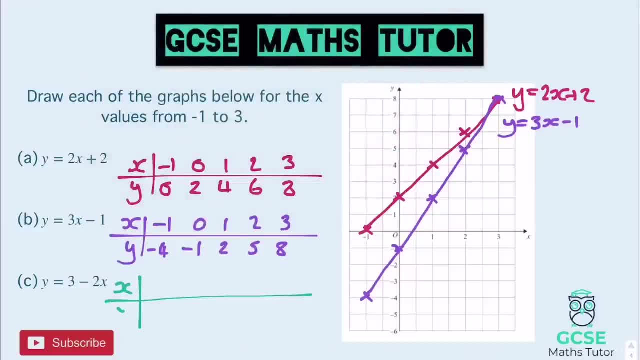 Might actually do some working out for this one. But let's have a look. We've got x and y And it goes from negative 1, 0, 1, 2, 3 again, So this time it's 3.. 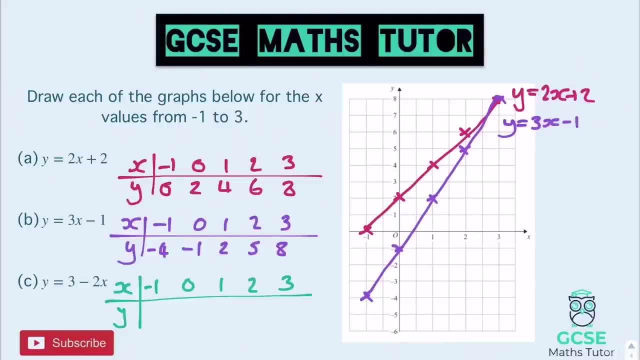 Take away 2 lots of x. So I'm going to do the working out for this one. So for that first one, there it's 3.. Take away 2 lots of negative 1.. So it's 3.. Take away 2 lots of negative 1.. 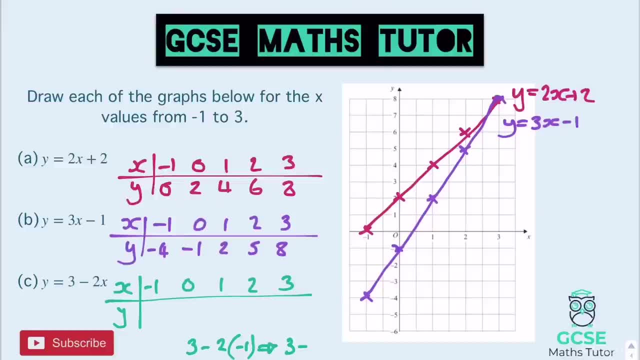 So that's 3.. Take away 2, lots of negative. 1 is negative 2.. So it's 3.. Take away negative 2, which is 3.. Add 2, which is 5.. So our first coordinate there is 5.. 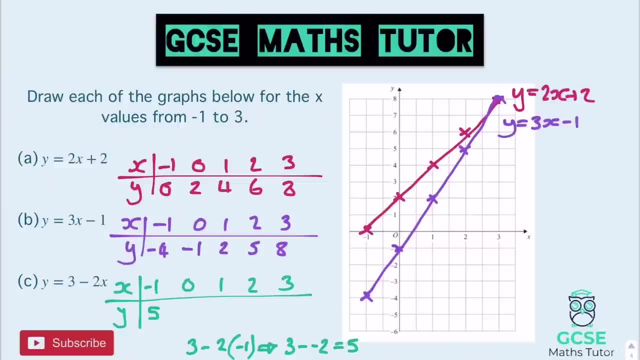 You've just got to be careful when you're subbing in these negative numbers into some slightly different looking equations. So negative 1 up to 5 is here, And then again doing the same for the next one, 3.. Take away 2: lots of 0.. 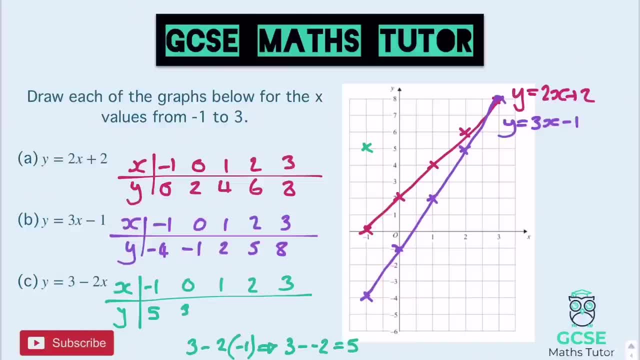 So 3.. Take away 0 is 3.. So 0 to 3.. There you go, And then you can see that this one is going down in twos, which is shown to you in the equation here. Negative 2x. 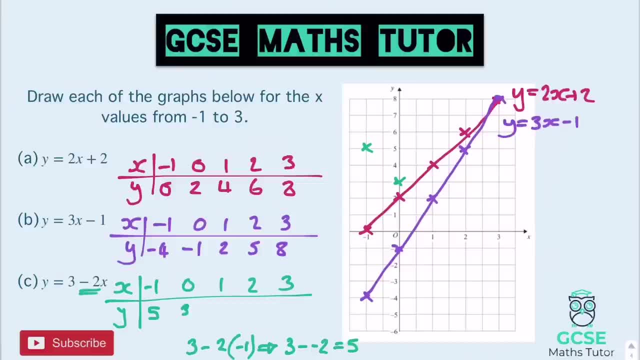 Now what you could do is actually rewrite this. You could rewrite it in the same format as the ones above. You could have written: y equals minus 2x plus 3.. And you can see there, look, we've got the y-intercept of 3 and the gradient of negative. 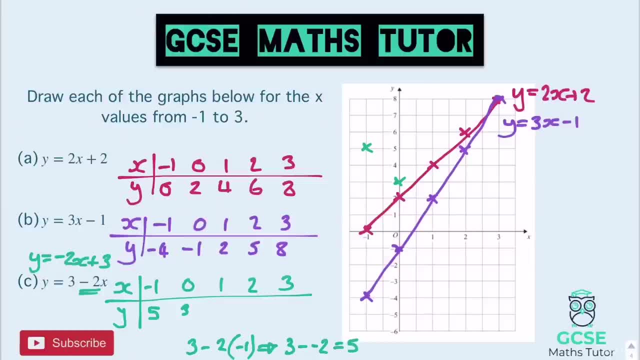 2. So when there is a negative gradient there, particularly when there's a positive y-intercept, it can be written in this other format here. So it's good to see this one and see another way that it can be written. But you can always rewrite them and rearrange them if you want. 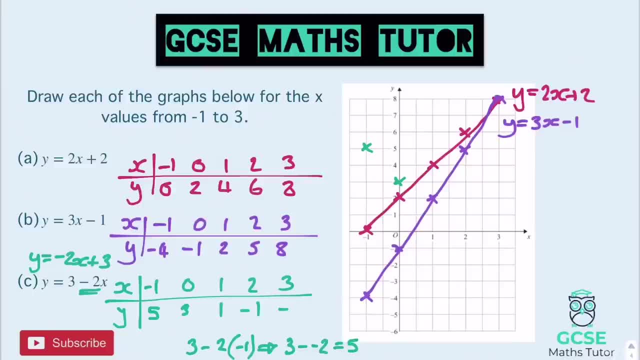 But it's going down in twos, so it's going to be 1 minus 1 minus 3. And we can just join them up. So 1 to 1 is there, 2 to negative 1 is here And 3 to negative 3 is there. 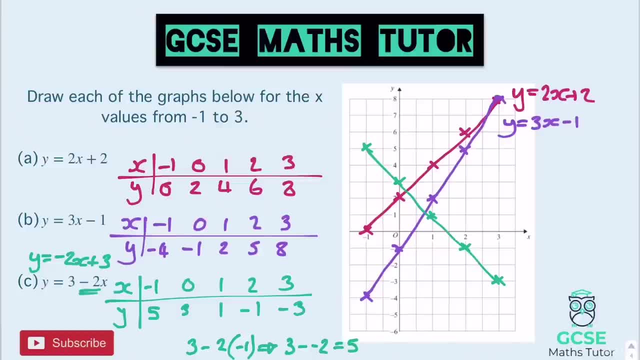 And again joining that up nice and neatly with a ruler and a pencil. There we go And we'll label that up. y equals 3 minus 2x. OK, So that's drawing these linear graphs. OK, If you're using the line equation, using a bit of a table there. 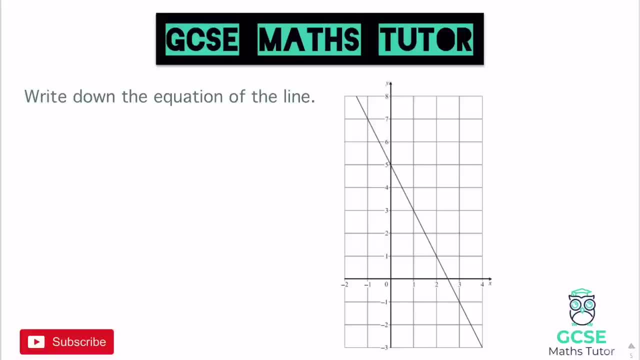 Let's have a look at something slightly different. OK, So in this question we are given a line already drawn on a graph And it says: write down the equation of the line. Now we know already that what the equation of the line is going to look like. 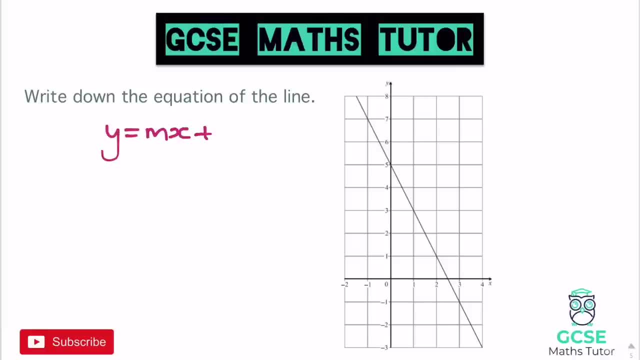 It's in this format: y equals mx plus c. Again, that's c being the y-intercept. Now we can see the y-intercept on the graph. It's over here, 5.. So for starters, I can actually just draw that straight in. 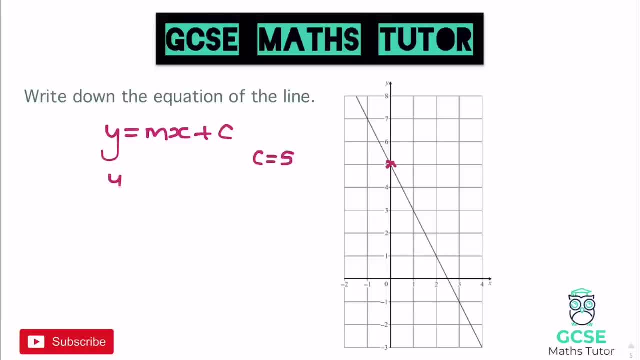 We can say c equals 5. And we can just put that in our line equation. So y equals mx plus 5.. All we need to figure out is what the gradient is. Now, if we have a look at this question, we've got to find some coordinates that we can actually see. 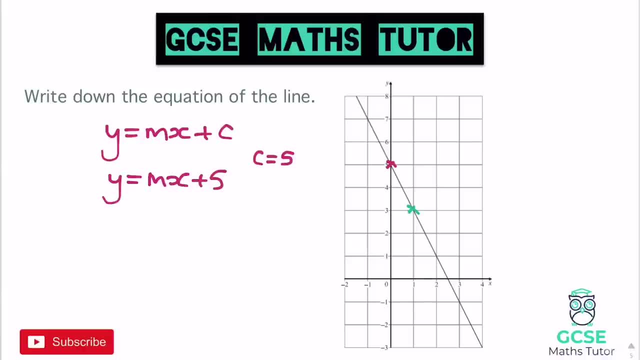 So here's another coordinate. that's on the line 1, 3.. Now if I want to find the gradient between these two points, all I have to do is draw a little right-angled triangle in So I can go across or down from this red point. 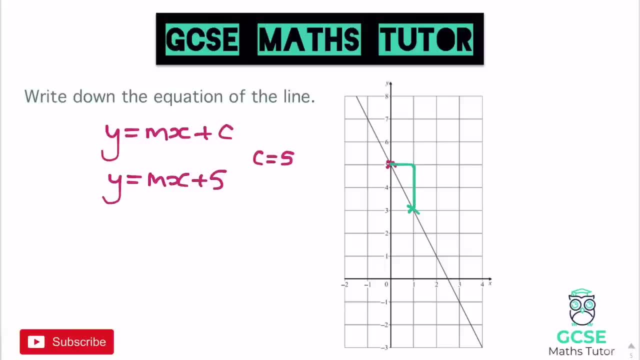 But if I go across and then down, I'm just going to say how big the movement is there. So that's a movement of 1 there And then that's going down 2. So I'm going to say that that's negative 2.. 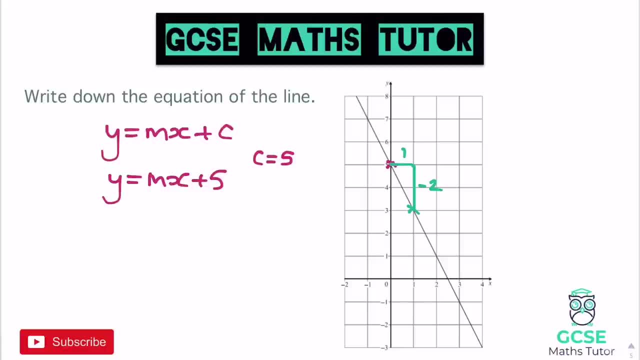 Now the equation to get the gradient. there's two different ways that you can look at it. You can have a look at it and use this little triangle. It means the change in, So it's the change in the y-coordinate over the change in the x-coordinate. 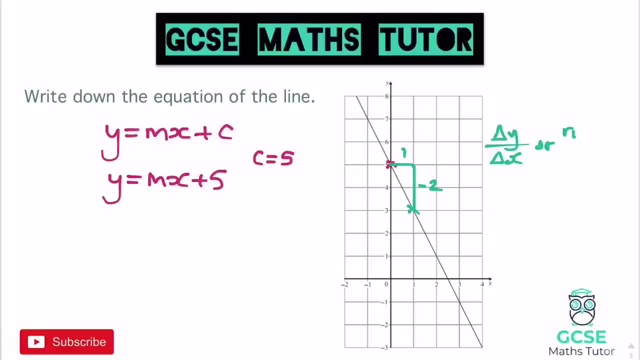 And it's sometimes referred to as rise over run. So you might know one of these two, But change in y over change in x or rise over run. Now, in this case, look the change in the y-coordinate. is this movement here going down? 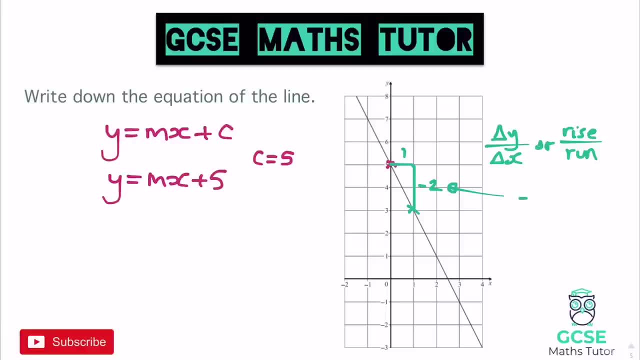 It's minus 2.. So that would be on the top of my little fraction here, minus 2.. And the run or the change in x is on the bottom. there is the 1 going across. So it's minus 2 over 1.. 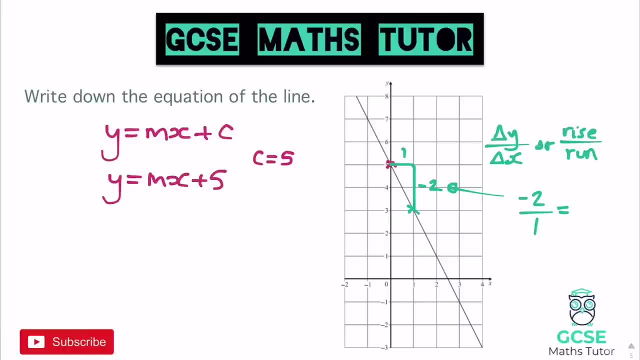 And minus 2 divided by 1 is negative 2.. OK, so my gradient here is negative 2.. So it's obviously sloping downwards, which is why it's going down. It's got a negative gradient, But that's what our gradient actually is for this question here. 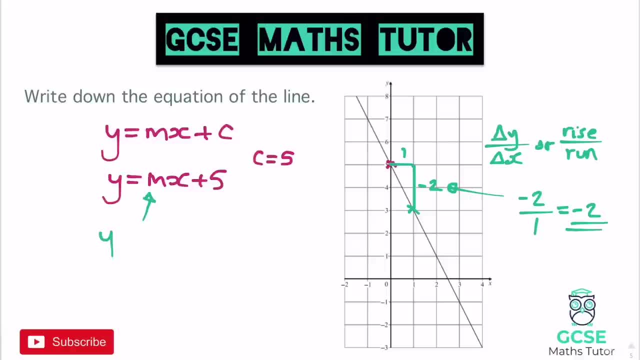 So all I've got to do is put negative 2 in place of m And we get y equals minus 2x plus 5.. Obviously, thinking about that last question that we looked at, you could actually write that as 5 minus 2x. 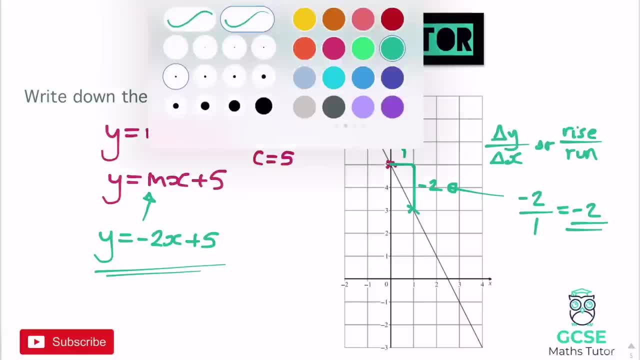 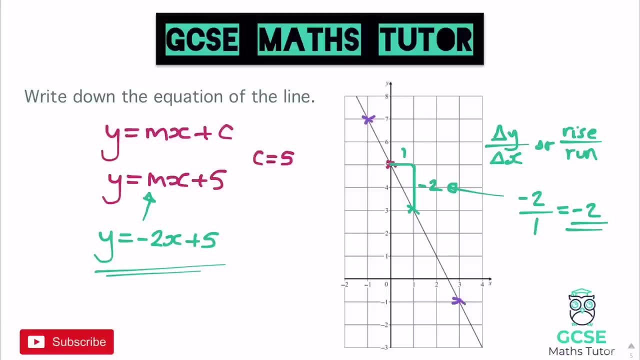 But you can write it in either way. It's absolutely fine to do so. Just a little side note: You can actually do these triangles as big as you want. If I picked some different coordinates, let's have a look. That one there and this one here, for example. 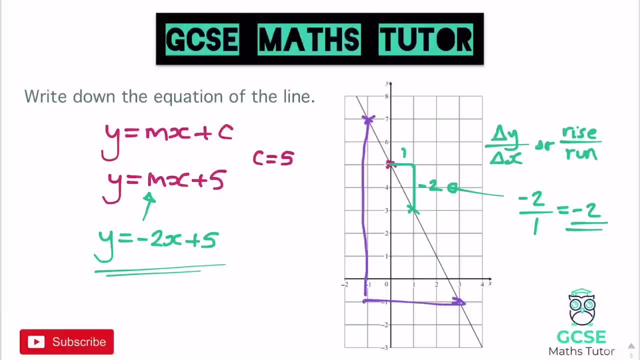 And if I was to go down instead and make a big triangle like this? let's have a look. My run there is 4. And my rise goes from 7 down to negative 1,, which is a movement of minus 8.. 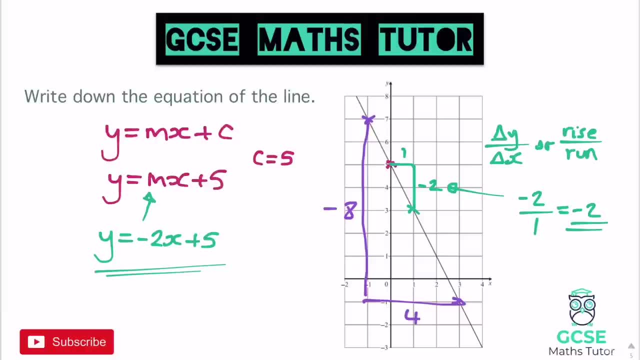 And if I did rise over run for this one or the change in y over change in x, it would be minus 8 over 4.. And minus 8 divided by 4 is minus 2.. So you can do this however you like, OK. 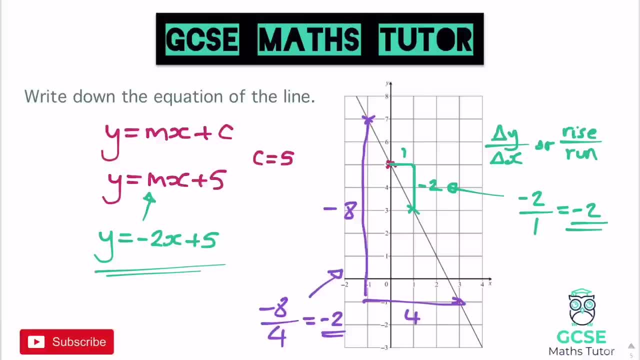 Because it's a straight line. it doesn't actually matter where you do the gradient from, It's just you just need to draw it in. Just read those numbers very, very carefully so you can get the correct gradient there Right now what we're going to actually have a look at. 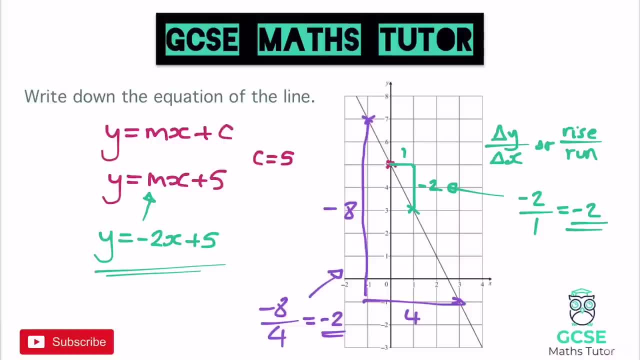 is doing this without a diagram, So just given the coordinates instead. So that's what we're going to move on to. Makes it a bit easier for you actually following along with the video. OK, but let's have a look at one of those. 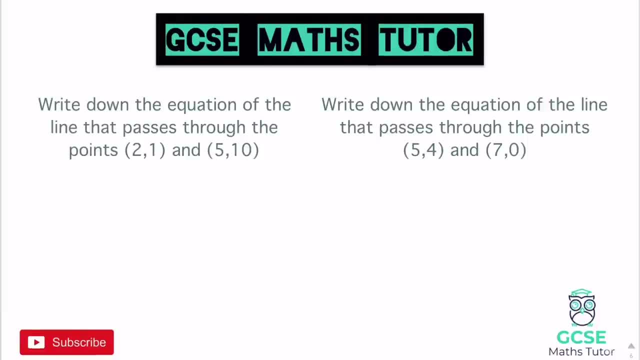 OK, so I've got two questions on the screen. I'm going to run through them both just so you can see the similarity in these sorts of questions. But I'm going to look at this one on the left to start with. So write down the equation of the line. 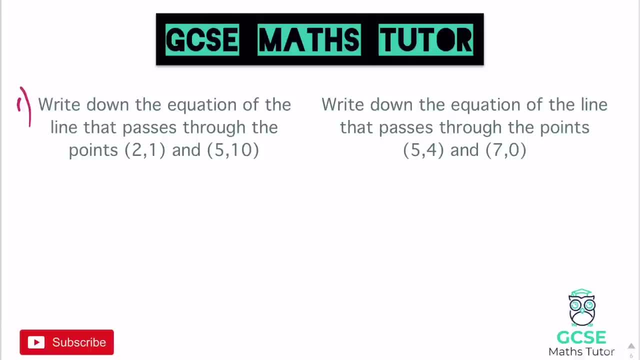 that passes through the points 2, 1 and 5, 10.. Now I don't need to go and try and draw a fancy graph for this. You can, if you want, just to help you visualise it. But I can actually do this just using the numbers. 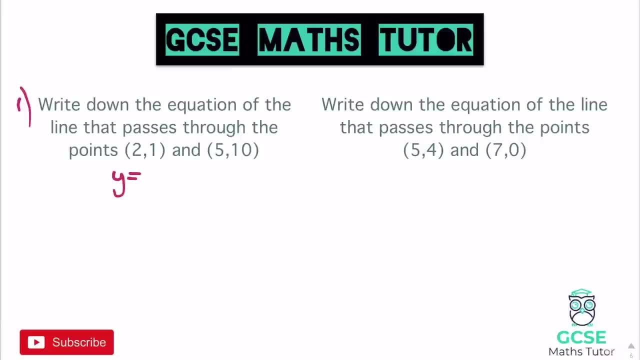 Now, first things first. I'm going to write down what the equation of the line is going to look like: y equals mx plus c. Now it's a slightly bit more complicated because we can't actually see the y intercept, so we do have to figure out all these pieces. 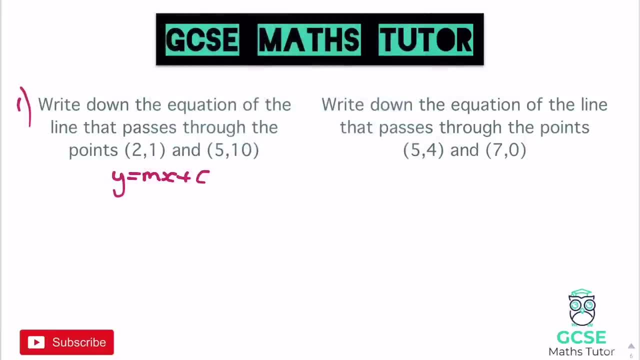 But in order to figure out the line equation, I've got to work out this gradient- Absolutely crucial to work out the gradient on this type of question. So, in order to work out the gradient, all I have to do is I have to look at these two coordinates. 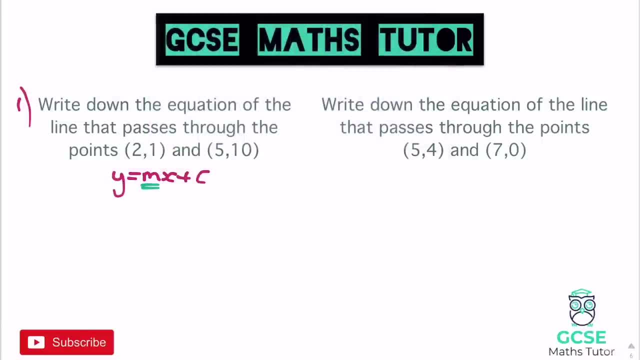 Now going from the first one to the second one. so by that I mean from this coordinate to 1, to 5,, 10,. I want to know what's the change in y and what's the change in x, because that's my little equation there. 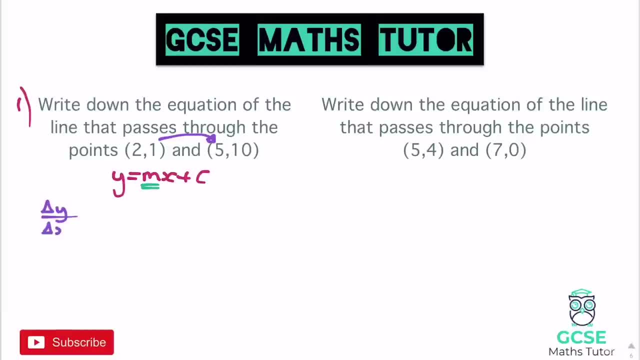 So I'm going to do the change in y. I'm going to divide it by the change in x. Now the change in y goes from 1 to 10.. So from 1 to 10 is positive 9, so I'll just put 9.. 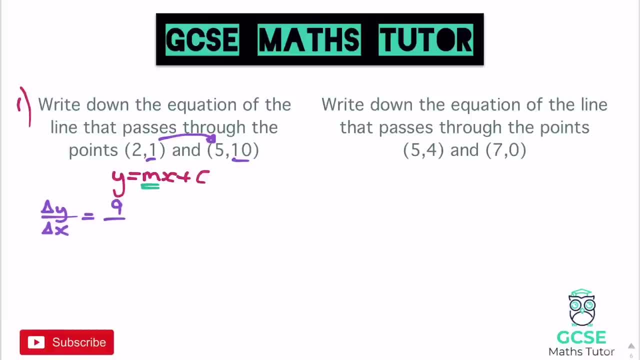 So that's my change in y. My change in x goes from 2 to 5.. That's positive 3. So from 2 to 5 is plus 3. So 9 over 3. And 9 divided by 3 is 3.. 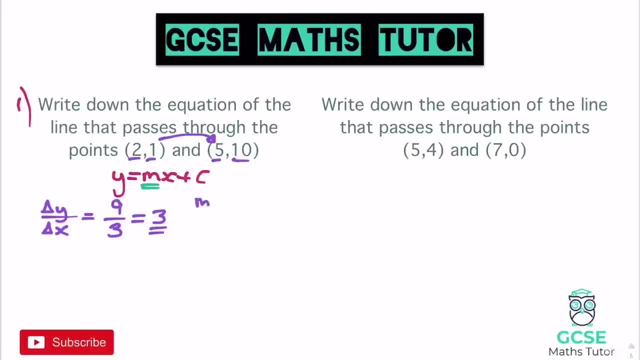 So my gradient is 3.. And it's always good just to write that down: m equals 3.. Now I can put that straight into our line equation: So y equals 3x plus c. But obviously now we need to work out the y-intercept. 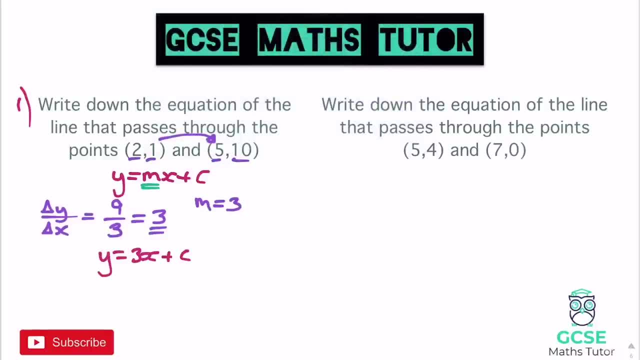 Now you have a choice at this point, because both of these coordinates- it says the line goes through, it passes through these points, so they're both definitely on the line. So if we pick either of these coordinates and sub them in, 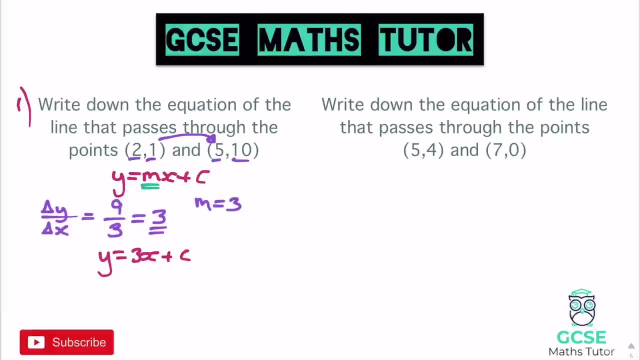 we've just got to make the equation balance, So I'm going to pick either one. Let's just go for the first one: 2, 1, although you can pick either. So the y coordinate's 1.. So let's put that into the equation. 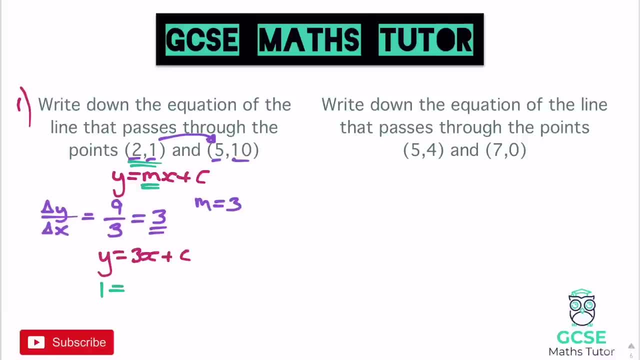 So 1 equals 3. lots of x, So 3 lots of that x coordinate, which is 2 plus c. There we go: 3 lots of 2 is 6.. So let's rewrite that again: 1 equals 6 plus c. 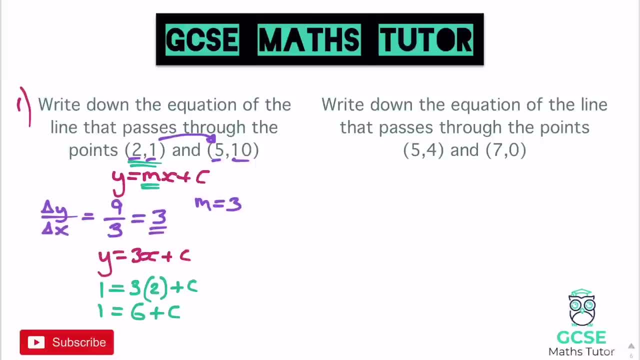 And hopefully you can see there that in order to make this side of the equation balance, c will have to be negative 5.. But you can subtract 6 from both sides there just to balance it like a normal single step equation And we get negative 5 equals c. 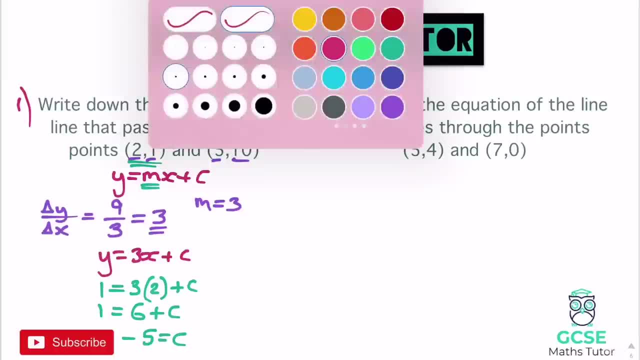 And then all you've got to do is completely rewrite the equation. So we've already got the equation here. Now we know what this c part is. We've got it down here: It's negative 5.. So we just put it all together. 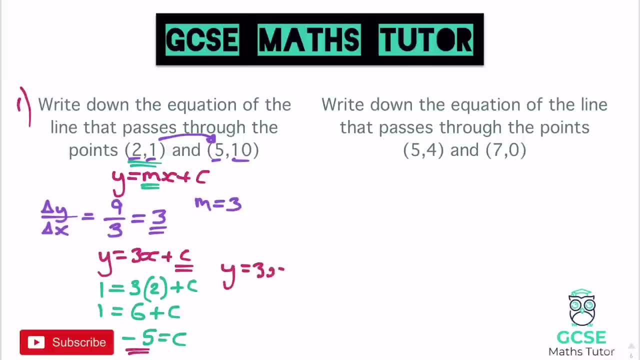 and we get: y equals 3x minus 5.. And there we go. There's the equation of that line: y equals 3x minus 5.. Okay, So we write down: y equals nx plus c. You use the change in y over change in x. 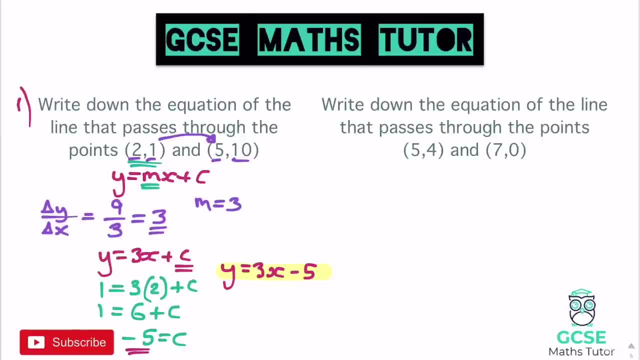 or rise over run to work out the gradient between the two coordinates. Get your gradient and then sub in either point to find your value of c, there the y intercept, and then just writing it all together. So quite a few steps here. 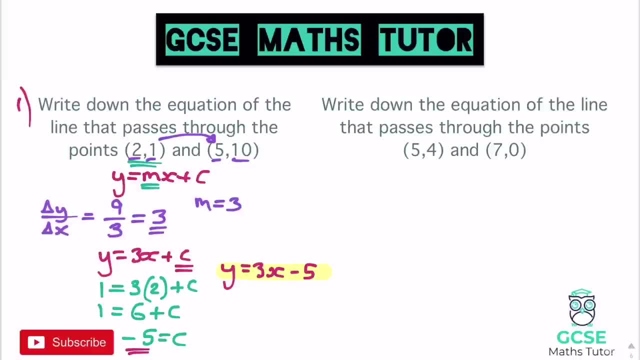 But there is one other thing, and that is just to make sure that we go from one coordinate to the other. So don't switch and swap. What I mean by that is, if you go from 2 here to 5, don't then go from 10 to 1.. 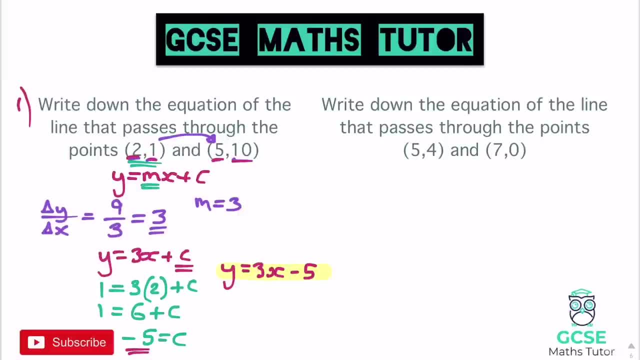 You have to keep it consistent between the two coordinates. Okay, So let's follow those same steps for this second question. It's exactly the same. I'm just going to follow my own steps. So again, write down: y equals mx plus c. 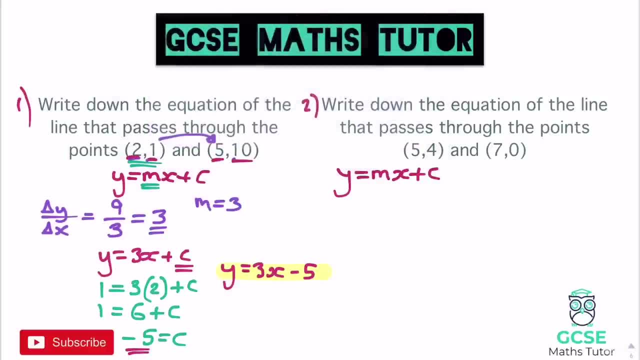 There we go. Let's have a look. We're going to work out m. So I'm going to go from this left coordinate to the right coordinate again And I'm going to figure out what the change in y over change in x is. 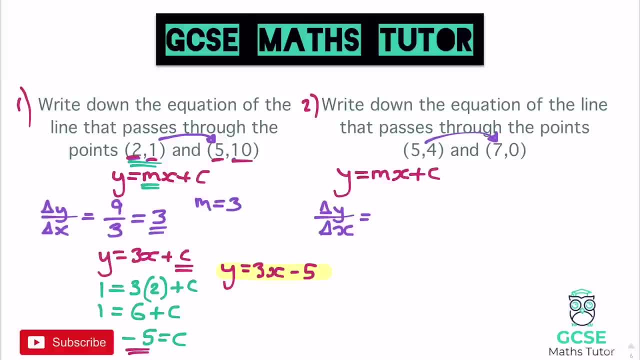 So for y it goes from 4 to 0. And that's a change of minus 4, negative 4, taking away 4 from 4 to 0.. The next one goes from 5 to 7. And that's a change of positive 2.. 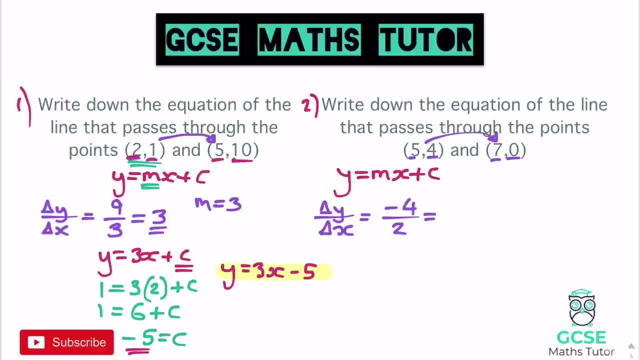 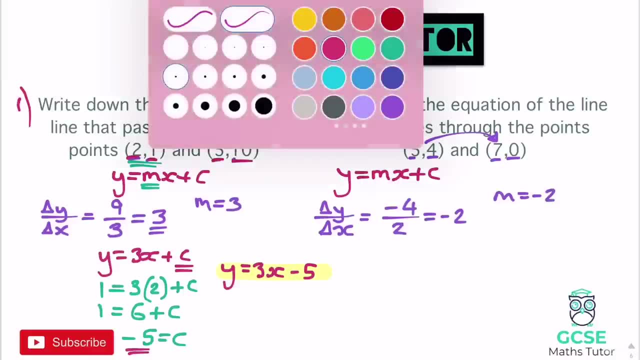 So over 2.. Now, negative 4 divided by 2 is negative 2.. There we go, So I'm just going to write down: m equals negative 2.. Again, just like before, let's put that into our line equation. 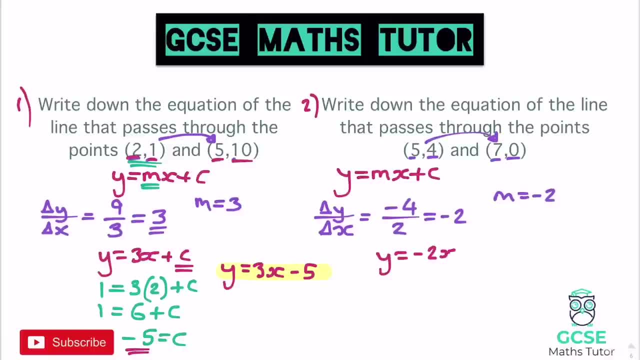 So y equals negative 2x Plus c, And then again pick a coordinate and sub it in. Now, just to make it a little bit different, let's sub the second one in this time Again, it doesn't actually matter. 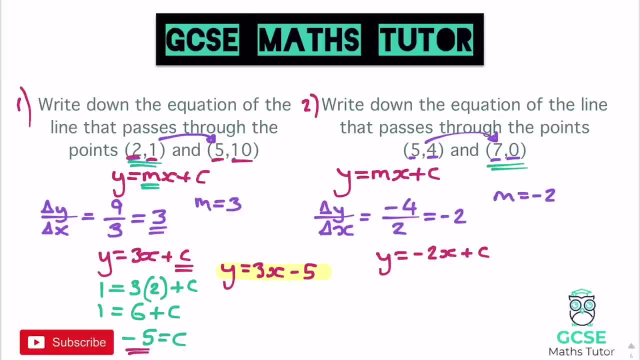 because they are both on the line. So let's sub that in. So y is 0. The y coordinate there, So 0, equals negative 2 multiplied by the x coordinate, which is 7, plus c. There we go. 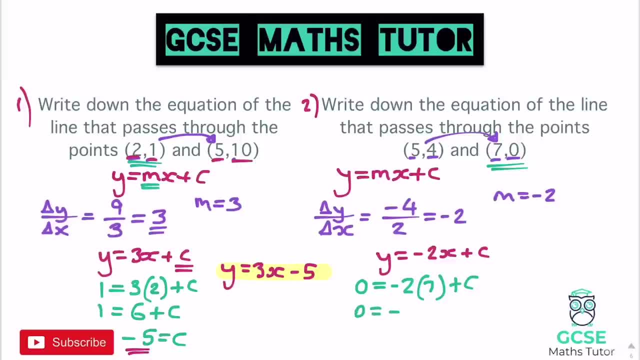 So 0 equals negative 2 times 7 is negative 14, plus c, And then add 14 to both sides. Let's try to balance this out. So 14 equals c, And then there we go, We've got our value of c. 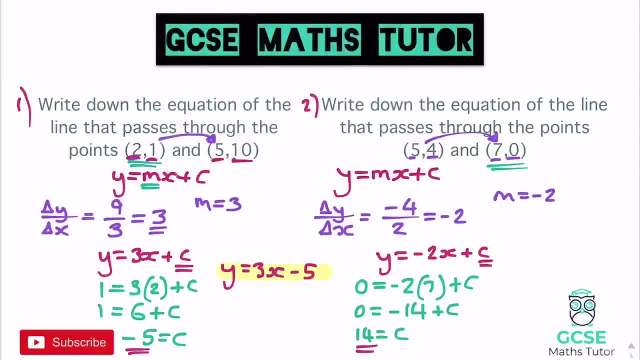 that we can plug back into our equation for c up here. So y equals negative 2x plus 14 there, As it is a positive 14, we obviously need to introduce that plus sign. So y equals 2x plus 14.. 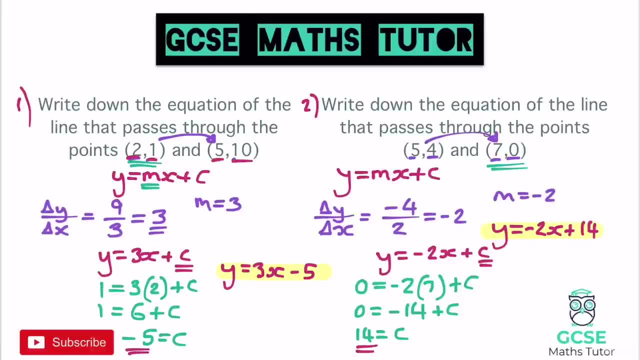 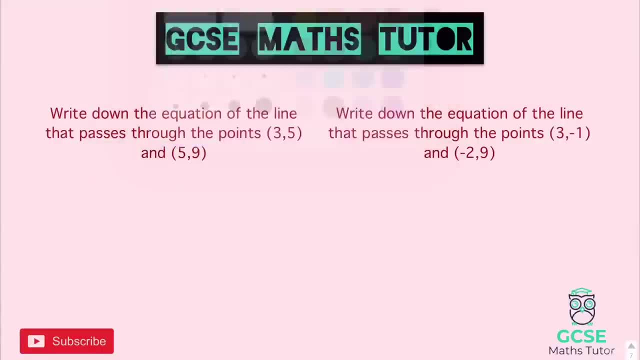 OK, So there's all the steps that you need to follow. Here's two for you to have a go at. So have a go at these two. Pause the video there. We'll be back in a sec, OK, So let's have a look. 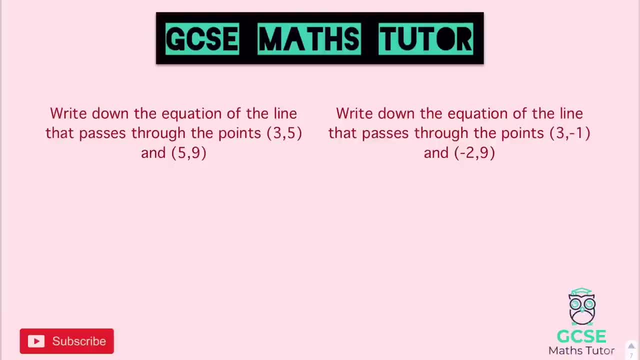 Write down the equation of the line that passes through these two points. So y equals mx plus c. I might skip a few steps in the working out. here We've got the change in y over the change in x. The change in y goes from 5 to 9,. 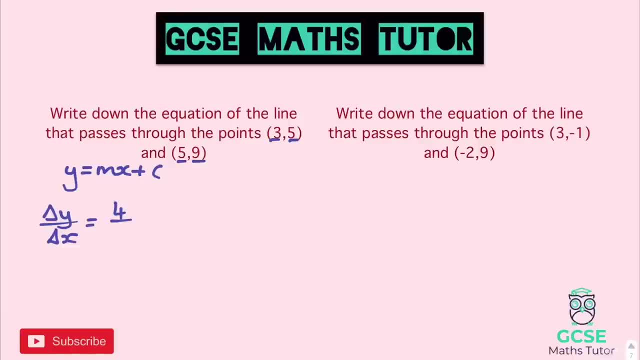 which is 4.. And the change in x goes from 3 to 5, which is 2.. And that gives us a gradient of 2.. So it's y equals 2x plus c. Pick a coordinate, So let's go with the first one here. 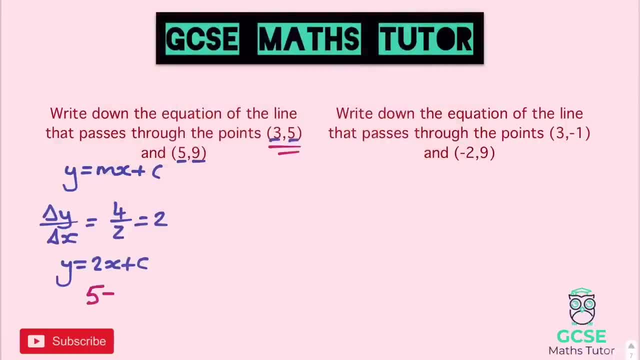 You might have picked the other one. So we have 5 equals 2 times 3, which is 6 plus c. Take away 6 from both sides. We get negative 1 equals c. There we go. Plug that in in place of c there. 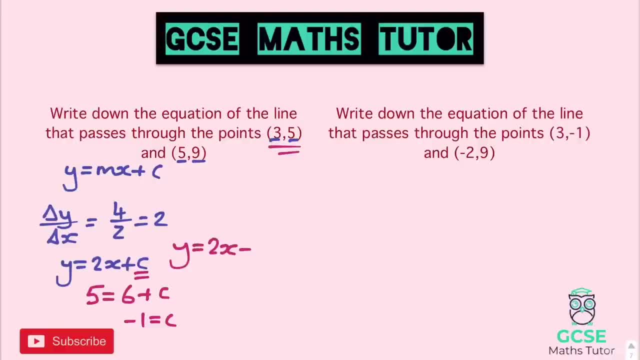 We get y equals 2x minus 1.. And there's our first line equation. On to the second one, I've already written down the line equation, so let's just work out the gradient. So change in y over change in x goes from: 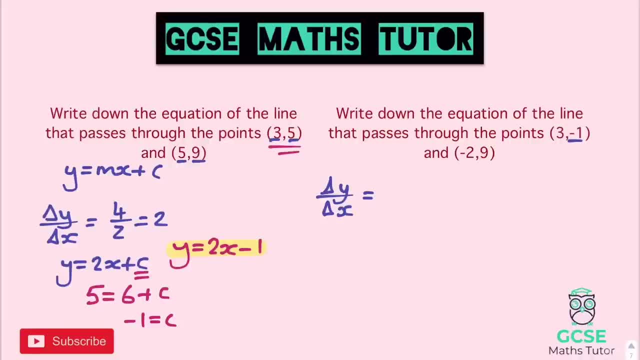 change in y. this time goes from negative 1 to 9.. Now that is a change of 10, positive 10.. From negative 1 to 9 is plus 10.. And then it goes from 3 to negative 2,. 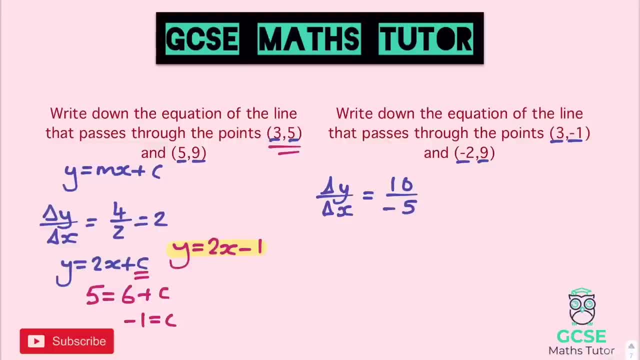 which is taking away 5.. 10 divided by 5 is 2.. 10 divided by negative 5 is negative, 2.. There we go. So y equals negative, 2x plus c, And now we just need to obviously sub our coordinates in. 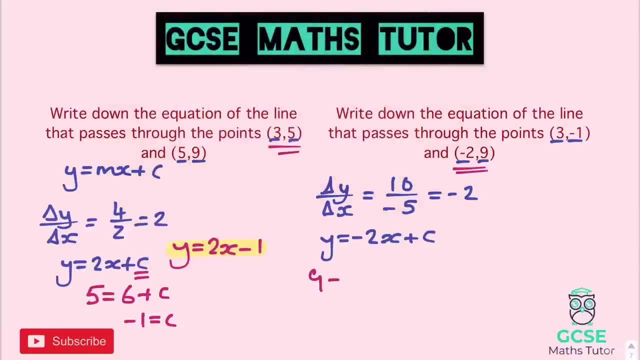 So let's go for the second one this time. So 9 equals negative, 2. Lots of negative 2.. I'll write this one down Plus c: Negative 2 times negative, 2 is positive 4.. So 9 equals 4 plus c. 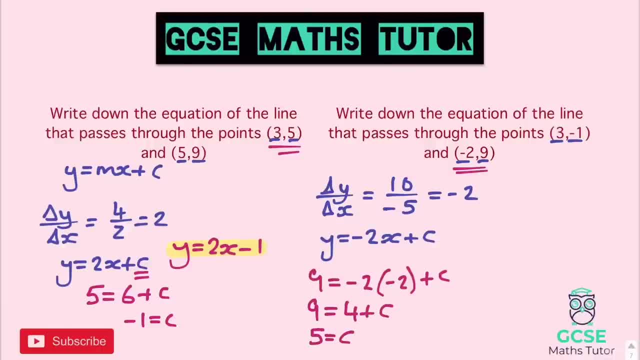 Take away 4 from both sides to solve it: 5 equals c or c equals 5.. And then write that into our line equation. here: in place of c, y equals negative 2x plus negative 2x plus 5.. 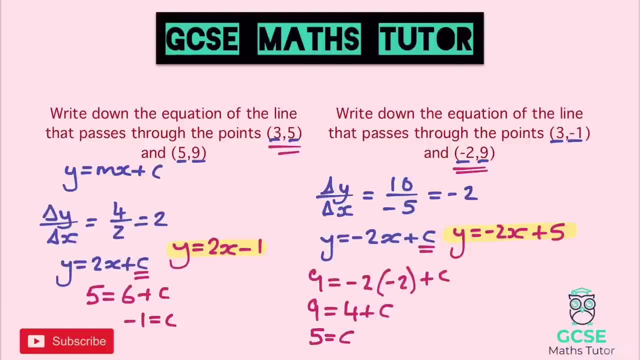 And again, obviously you could rewrite that as 5 minus 2x, but that's fine, just to leave it like that, Right? let's have a look at a slightly harder one. Okay, so a slightly harder question here, and you'll see why when we work this one out. 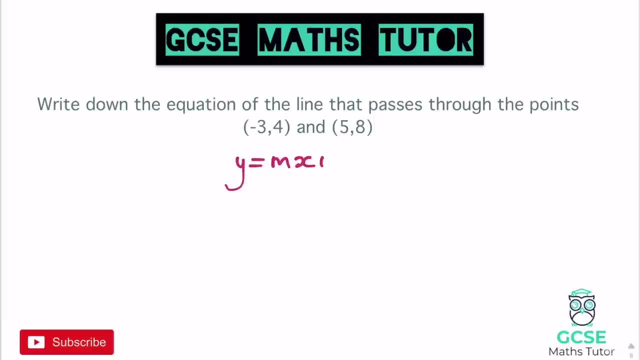 So we've got y equals mx plus c And we're going to work out the equation of the line between these two points. So the change in y over the change in x, Let's see what we get. So from 4 to 8 is positive 4.. 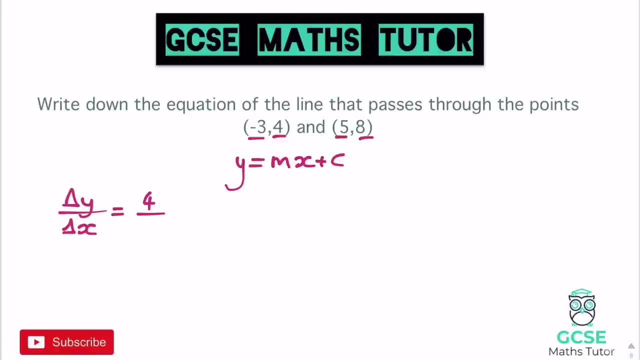 And from negative 3 to 5 is a movement of positive 8. So it's 4 over 8.. Now we've got a fraction here. We can simplify that. So divide the top and bottom by 4. And we get 1, half okay, or 0.5.. 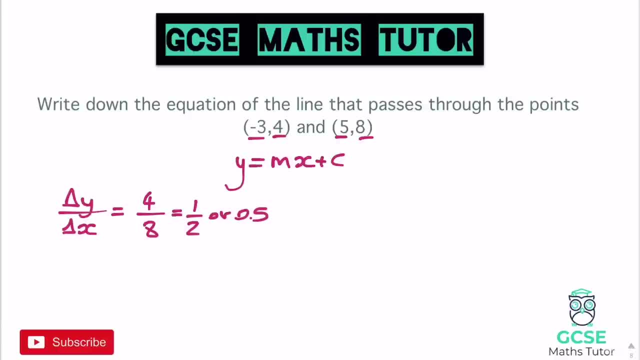 Now, it doesn't matter whether you use fractions or decimals here. It's completely up to you which one you prefer to use. I think I'm going to use it as a decimal. I'm going to keep it as 0.5.. And let's put that into our line equation. 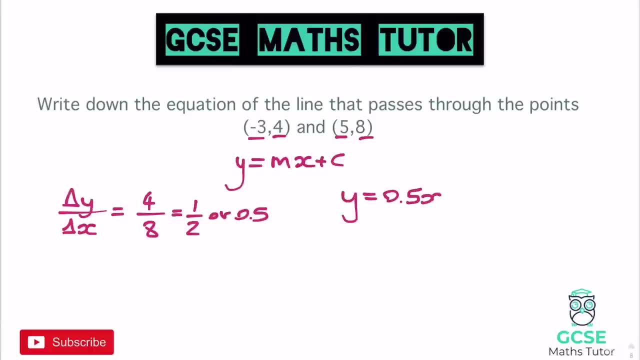 So y equals 0.5x plus c. Right, let's pick a coordinate. I'm going to go for this one here, just because it's got two positive numbers in, But it's completely up to you. It doesn't actually matter which one you use. 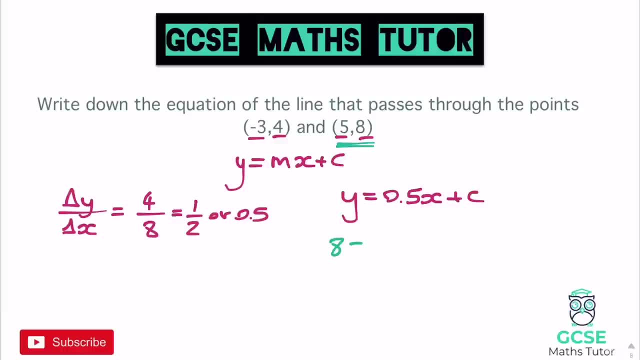 So let's sub that in, So we have 8 for y. So 8 equals, We've got 0.5, lots of the x coordinate there, which is 5, plus c. There we go, So 0.5 times 5, or half times 5.. 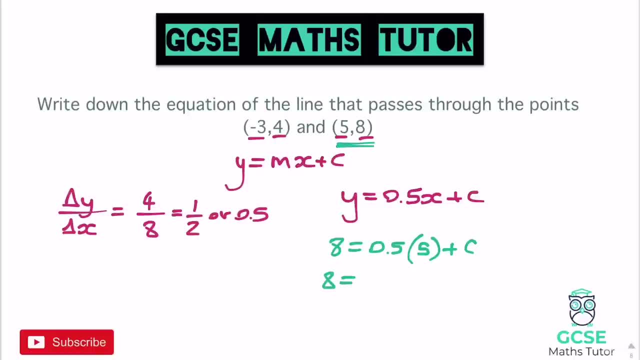 Let's have a look and see what that is. So we get 8 equals 0.5 times 5 is 2.5. And then we get 0.5.. A few times by a half, it just halves the number. 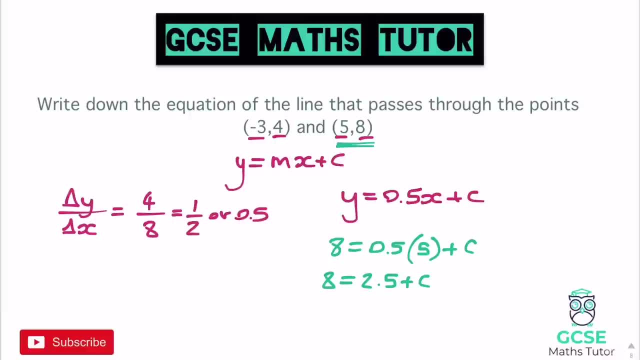 So 2.5 plus c, And then we need to subtract 2.5 from both sides to figure out what c is there. I mean you can just use logic: From 2.5 up to 3 is an extra half. 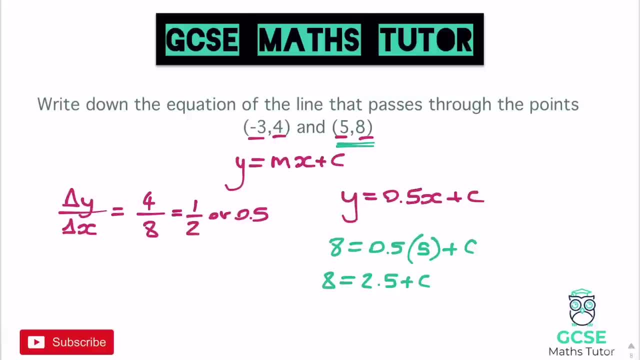 And then it's an extra 5 to get to 8.. So it's 5.5.. And if we subtract 2.5 from 8, we get 5.5 equals c, And then we can plug that in place of c. 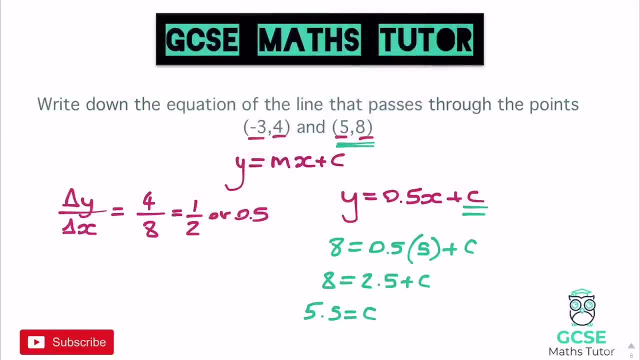 up in our line equation there. OK, so let's write that out. We get y equals 0.5.. So y equals 0.5x plus this 5.5.. There we go, And there is our line equation. 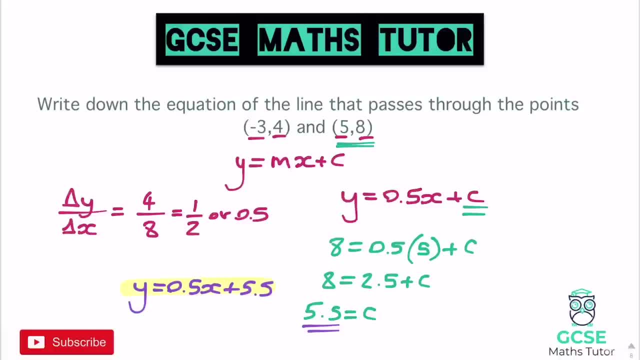 So y equals 0.5x plus 5.5, which again you could write as a fraction if you want. So whatever value you get for the gradient, obviously just treat it as a fraction or a decimal And just obviously careful on this step, right here. 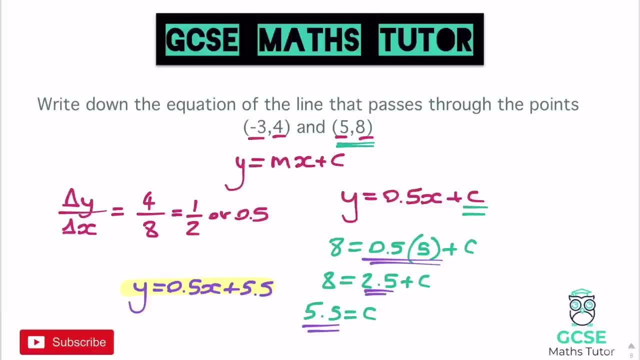 Just when you multiply those to get this value of 2.5, whatever that decimal multiplication is. be careful with that. OK, so here's one for you to have a go at. OK, so it says: write down the equation of the line: 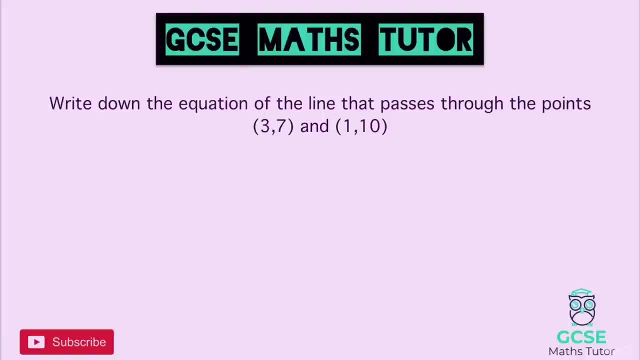 that passes through these two points. So do your change in y over change in x, Work out your gradient. Be very careful because it is going to be a decimal. Just be careful when you multiply it, when you sub those coordinates back in. 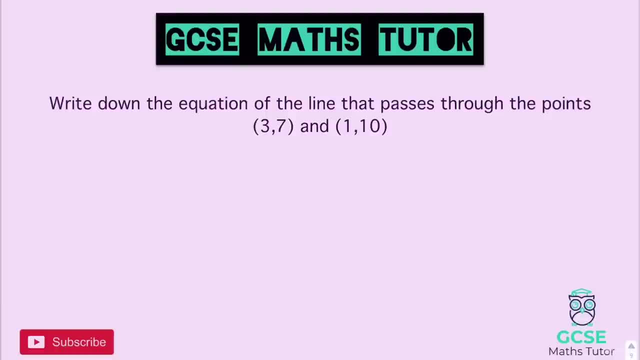 But pause the video there, have a go, and we'll go over the answers in a sec. OK, so let's have a look. Let's write down the equation of the line, So y equals mx plus c, And let's work out the change in y over change in x. 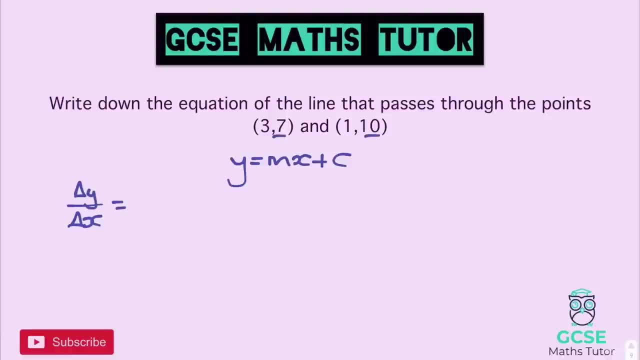 Right, so it goes from 7 to 10,, which is 3.. And it goes from 3 to 1,, which is negative 2.. Right, not the nicest one here. So that is negative 1.5.. 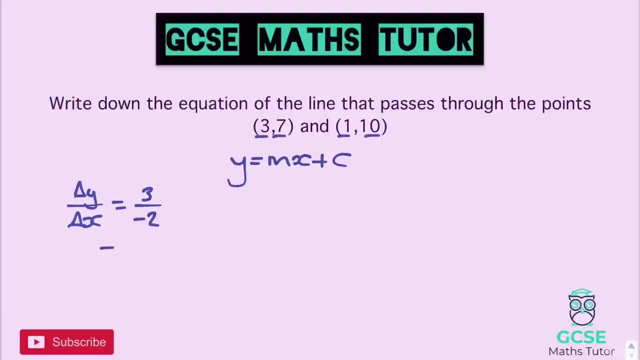 3 over 2 is 1.5.. You can leave it as a fraction if you want, But I'm going to write that as negative 1.5.. There we go. So that is the value of my gradient. m equals 1.5.. 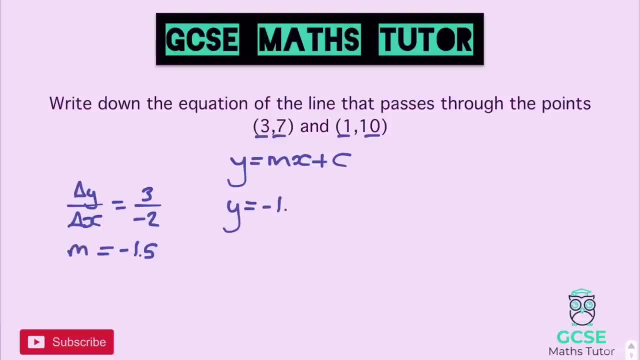 And let's put that in: So y equals negative 1.5x Plus c. Right, so now we just need to pick a coordinate Again. you can pick either 1 here. I think it might actually be easier just to go for the 1 and the 10.. 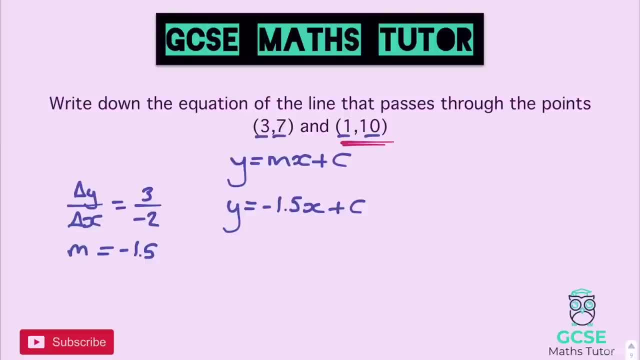 Although you could go for the 3 and the 7.. The 1 and the 10 is definitely easier there, because timesing 1 by negative 1.5 is a bit easier than timesing 3 by negative 1.5.. 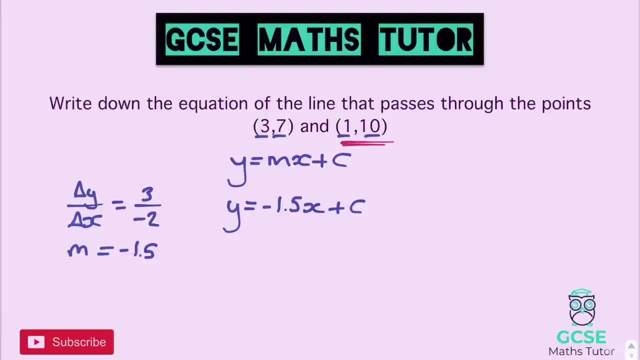 But let's just go for this: 1 and the 10. So 10 is y. So 10 equals negative 1.5 multiplied by 1 plus c, Right? So 10 equals negative 1.5 times 1 is negative 1.5 plus c. 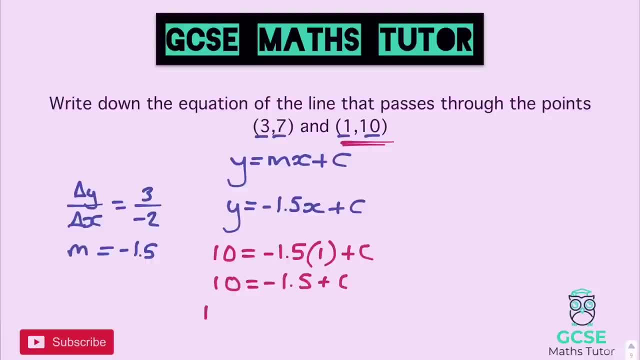 And then add 1.5 to both sides to balance this out. So we get 11.5 equals c, And then we can just write our line equation there. We can put that in place of the c And we're finished. 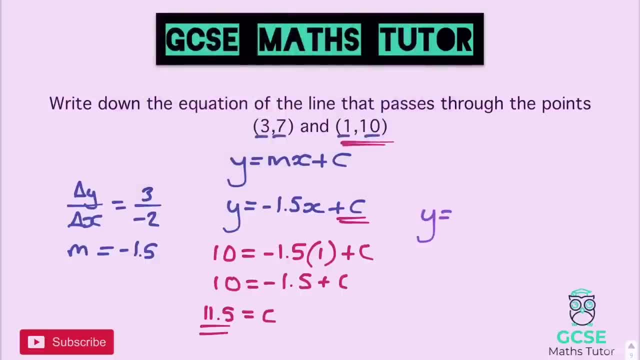 So let's write that out. So y equals negative 1.5x plus 11.5.. There we go. Just a little side note, just in case you did use the other coordinate. look what would happen in that case. Well, if we sub those in, 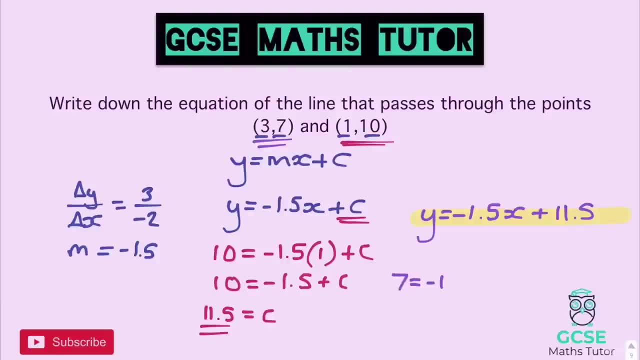 we get 7 equals negative 1.5 times this times 3 plus c. There we go, So we have 7 equals negative 1.5 times 3 is negative 4.5. And if you add 4.5 over to 7,, 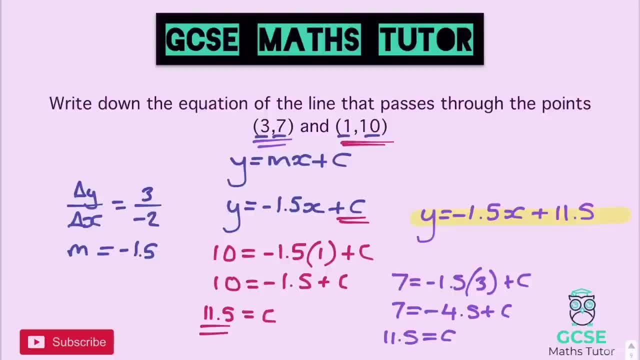 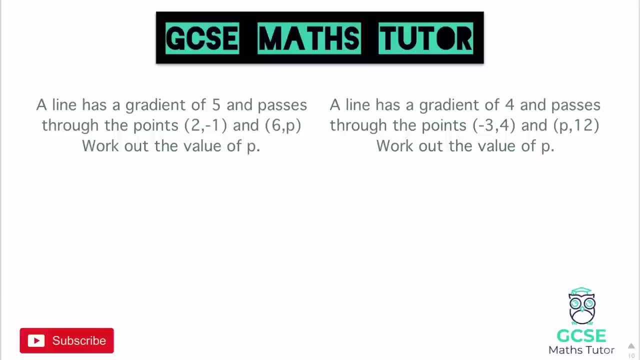 you get 11.5 equals c And you get the same value of c there, obviously, to plug that into your line equation, Right, OK, Let's have a look at one more thing before we finish here. OK, So I've got two questions here. 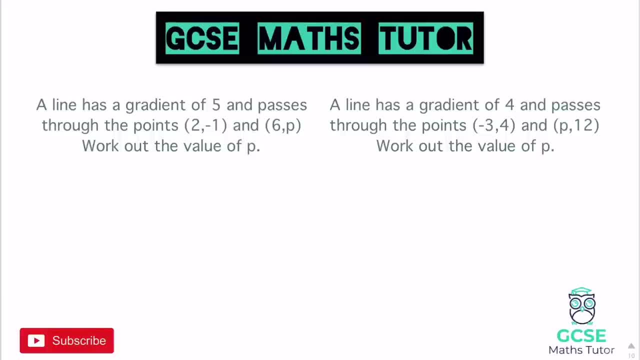 It says a line has a gradient of 5 and passes through the points 2,, negative 1, and 6p. Work out the value of p And we've got another one that's very similar over there. If you have a look. we've got this value of p in this second equation for the x coordinate. 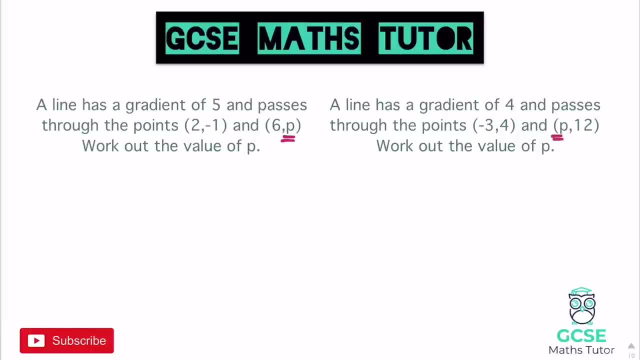 And in this part here it's in the y coordinate Right. So what you need to do on this sort of question here is have a think about what you can do. So you know y equals 0x plus c. You know that you need to find the gradient. 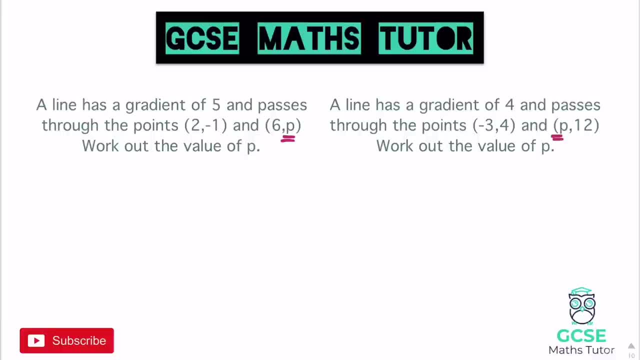 which is given to you in this point, So you can definitely write the equation of a line. You know how to find the full equation of a line now because you can sub one of the coordinates in And in both instances here there is one coordinate definitely given to us. 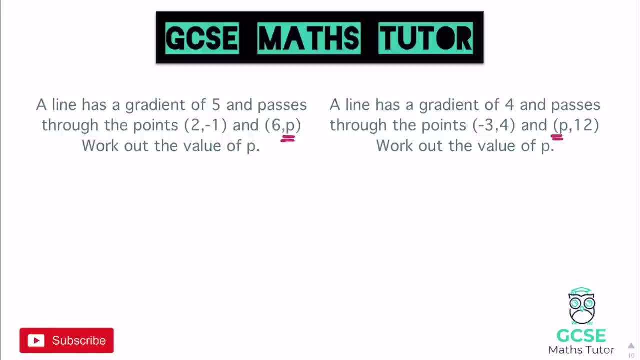 So you can definitely get the equation of a line And then you can think about, once you have the equation of a line, how are you going to find these missing pieces in the coordinates? OK, And that's just going to come down to making sure that, once you have the equation of a line, 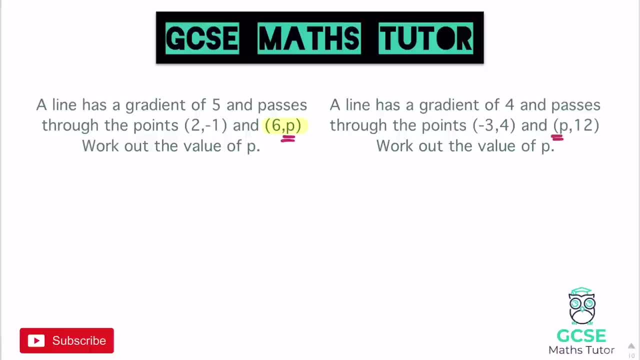 you can sub in one of the points here. So in this case you can sub in 6 in place of x, And on the second question over here, you can sub in 12 there in place of y. So both slightly different. 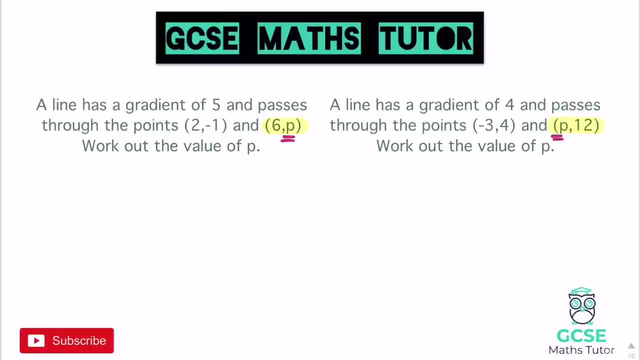 OK, But what I want you to do is to have a go. This is your last sort of questions to have a go at, So I encourage you just to see how far you can get on both of these, See if you can find out what these values of p are. 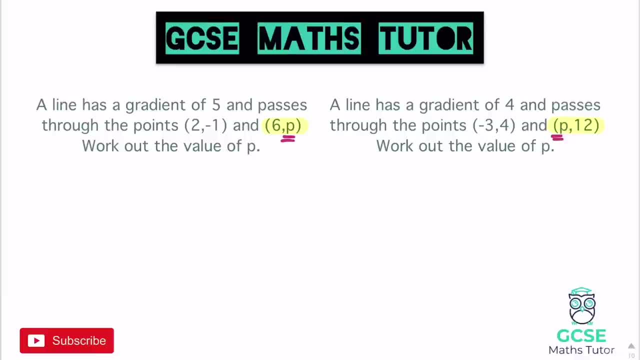 That's a little bit of a problem for you. So have a go See what you get. Pause the video there And we'll go over the answers in a sec. OK, So the first one. The line has a gradient of 5.. 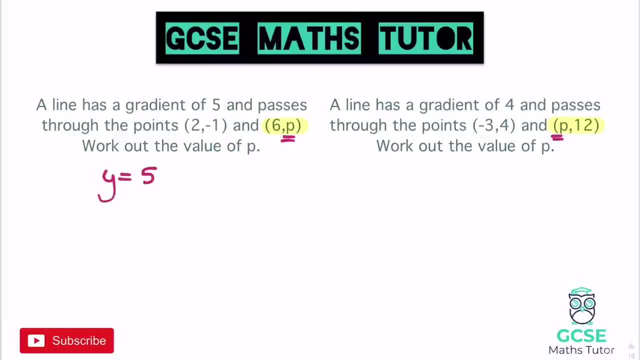 So straightaway we can write out: y equals 5.. Now y equals 5x plus c. It then gives us one of the points here, So 2, negative 1.. So if I put 2, negative 1 in, let's have a look at what we get there. 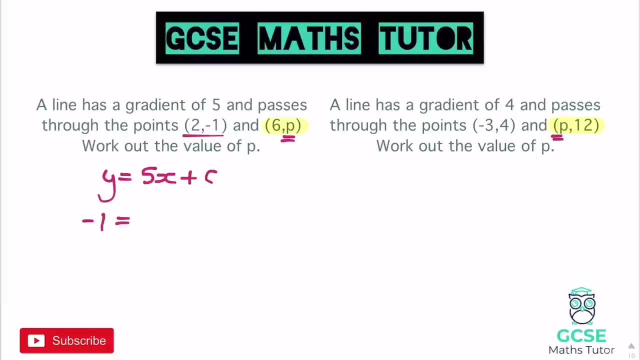 We get minus 1 equals 5 times 2 plus c. OK, So now that we've got that, we can have a think about how we're going to move forward from this. So, just like before, I'm going to actually just get the value of c. 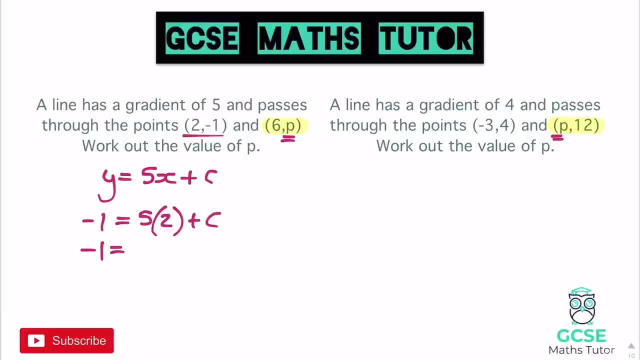 So I have minus 1.. Y equals 10 plus c. There we go. And if I take away the 10 here, we get negative 11 equals c. Right, So I can write the equation of the line. now Let's actually write the equation of the line. 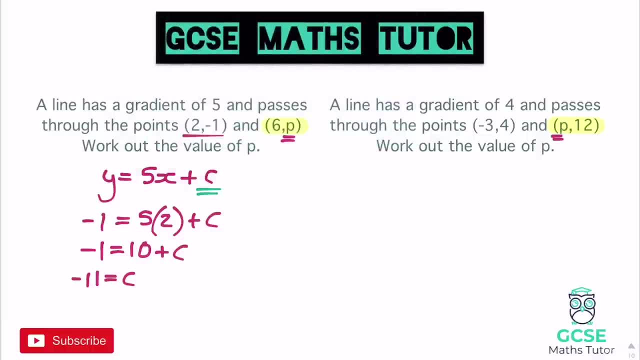 So where is our starting bit? There we go. That's where we're putting c, So we get y equals 5x minus 11.. Now, obviously, up to this point, you've actually done all of these bits of maths. on the previous questions. 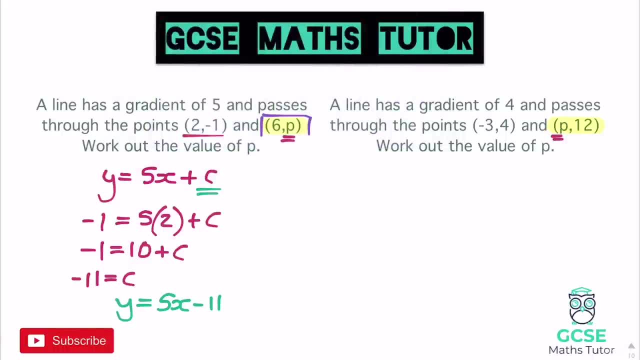 So to actually finish this off, look, I'm just going to focus now on this coordinate. If it's on the line which it says it is, it passes through that point. If I sub it in, all I need to do is make sure the equation balances. 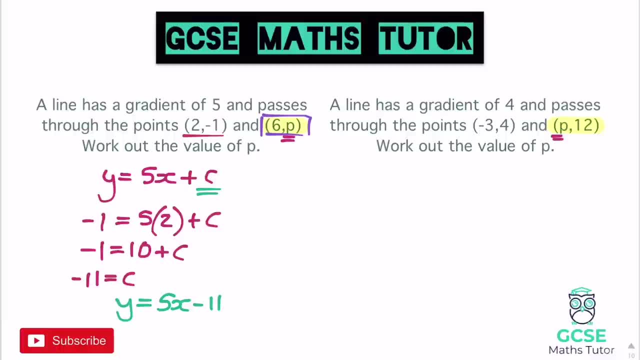 So I can sub 6 in place of x. So if we sub that in, look, if I put 6 in place of this x, here we get y equals 5, lots of 6 minus 11.. Let's bring this up here. 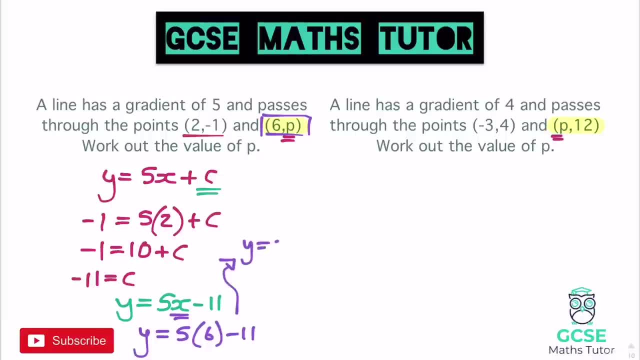 5 times 6 is 30. So y equals 30 minus 11. And that means y equals 19.. And there we go. So the y coordinate has to be equal 19,. finishing that one off. Now there are other ways that you can do this. 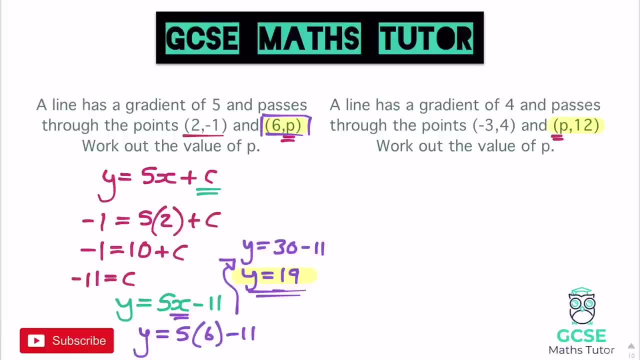 You can actually draw a little diagram and you can use the sort of like the little triangle idea- your eyes overrun. But I just think using this idea here really does help with the progression of this topic, rather than looking at little tricks for every different type of question. 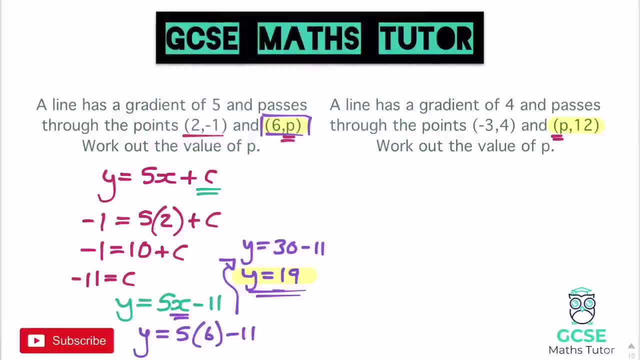 Just like I mentioned on the very first ones, a little trick you can do when drawing a line. I think if you just keep it consistent- using y equals mx plus c and really understanding how to use that, it does help as you progress onto those higher level topics within this. well, the subtopics within this topic of coordinate geometry. 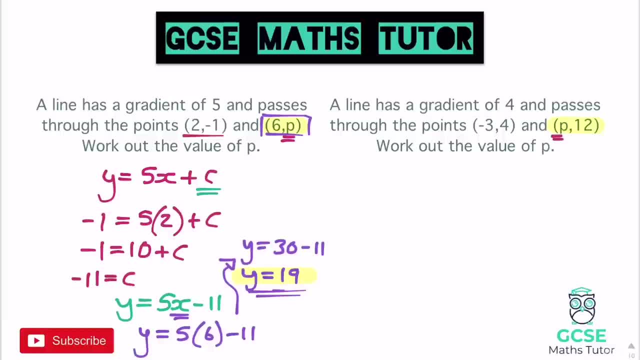 So let's have a look at the next one. So this one has a gradient of 4.. So again, y equals 4x plus c, And again we've got a coordinate we can sub in. So I'm going to sub this coordinate in. 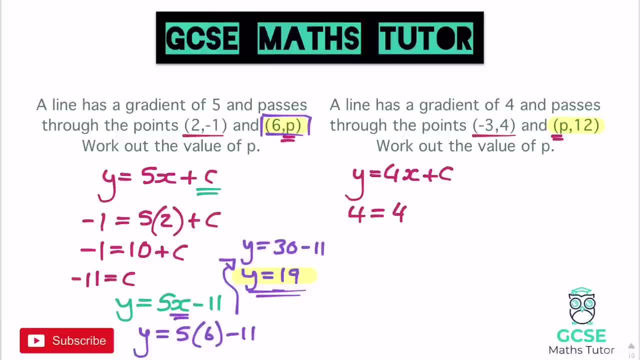 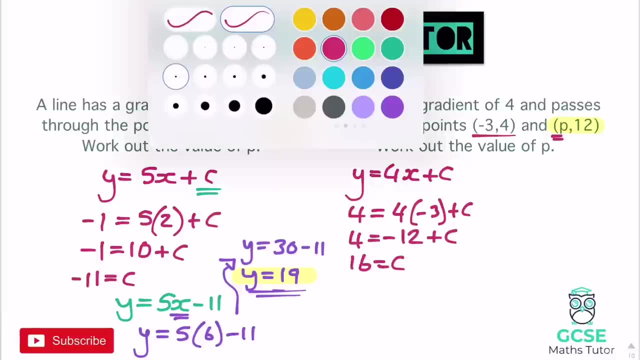 So y is 4.. y equals 4 lots of negative, 3 plus c. So 4 equals 4 lots of negative. 3 is negative 12 plus c. Add 12 to both sides, we get 16 equals c. 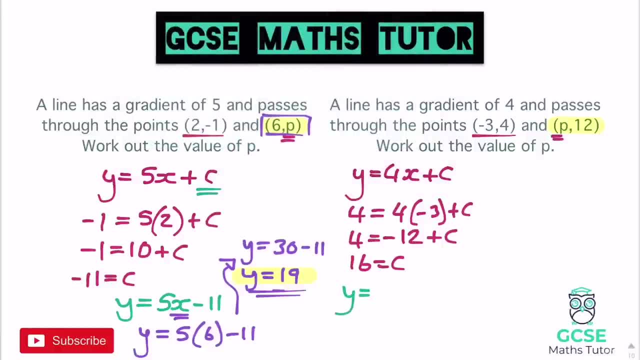 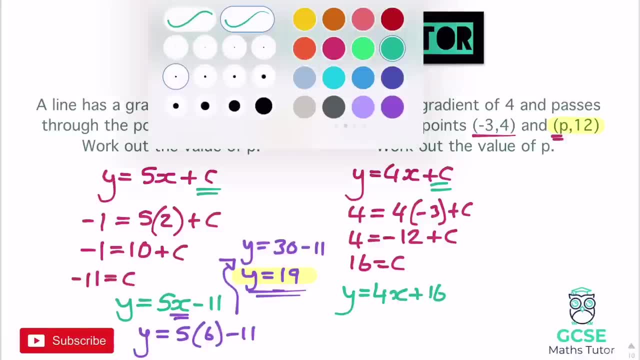 And if we write the line equation out just like before, we have y equals and that's our c that we're putting into there 4x plus 16.. Right now we can actually start to tackle this next one, this coordinate up here. 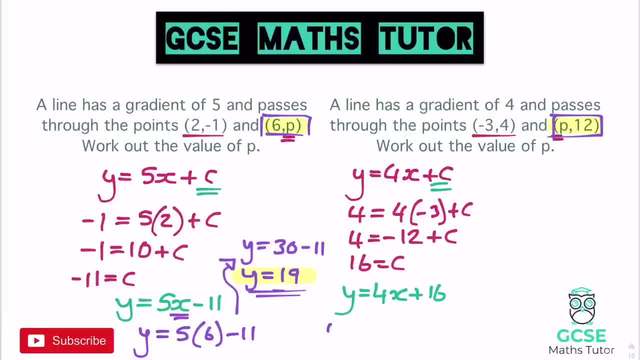 We've not got the x coordinate this time we've got the y coordinate, But we'll put that in the place of y. So we have 12 equals 4x plus 16.. And then hopefully you recognise that as just an equation to solve. 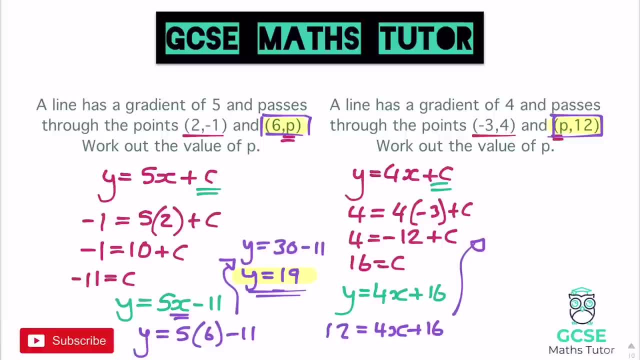 So again, if I bring that up here, we'll subtract 16 from both sides, So we get negative 4 equals 4x And then divide both sides by 4. And we get negative 1 equals x or x equals negative 1..